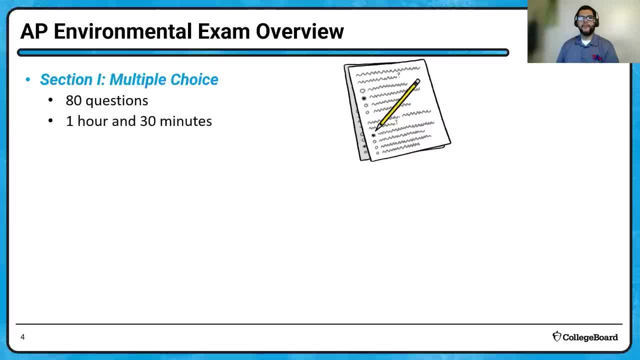 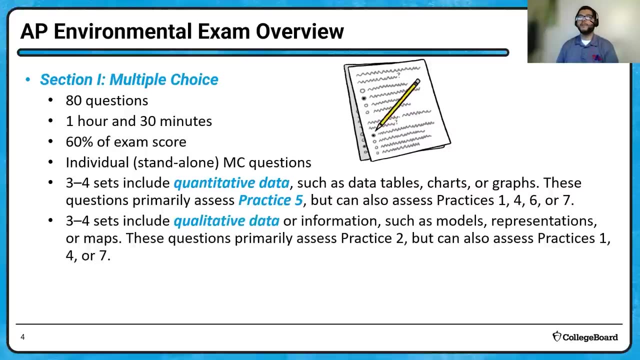 We went over that in video one with 80 questions, hour and a half, roughly over a minute per question, 60% of our exam score And of course we're going to have standalone and data sets and qualitative sets. So if you have not had a chance, please review video one so you can look at the different types of multiple choice questions. 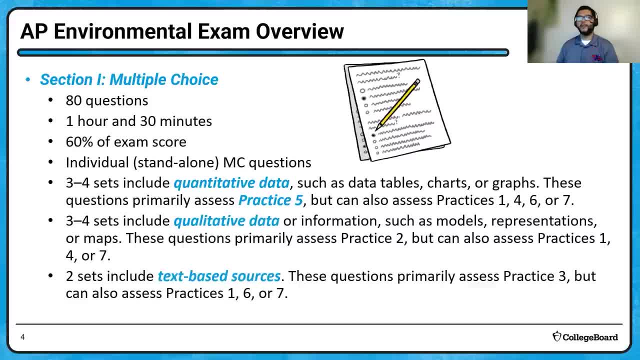 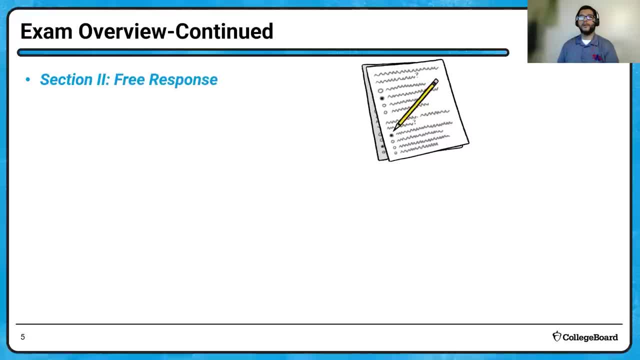 And we also have text based questions that are only. And then, of course, free response section. The next video will be covering a lot of this. Miss Faster will be going over those And that's going to be three questions hour and 10 minutes- about 20 minutes per question. 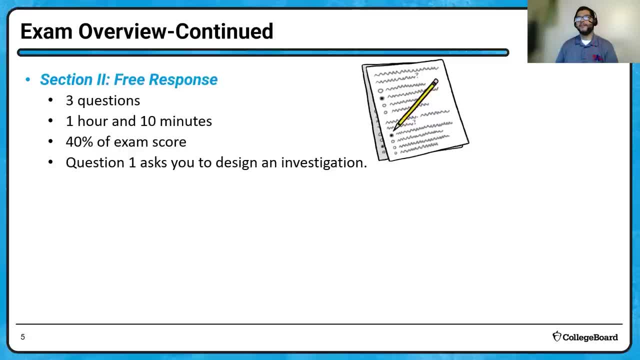 That's 40% of your score, And it's going to ask you to design an investigation always and then analyze a problem with a solution and then do the same with calculations. That's actually the type we're going to be looking at today. 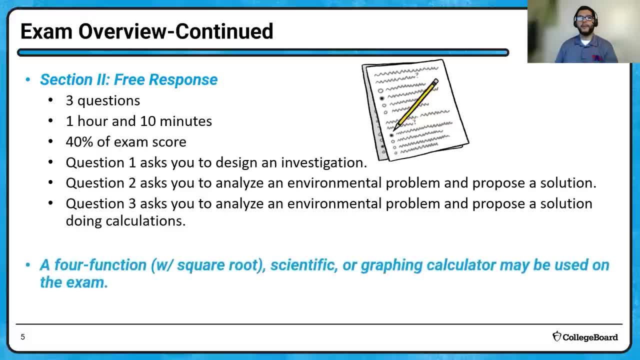 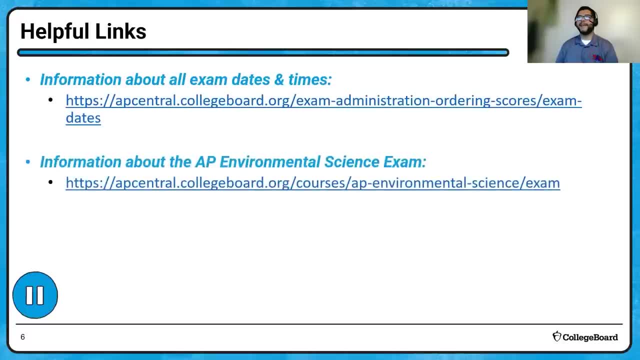 So you'll get a chance to look at that as well, And then you do get a four function calculator for those Calculations. So here we have some links for you to help looking at the AP exam dates and the environmental science exam for in general and for students. 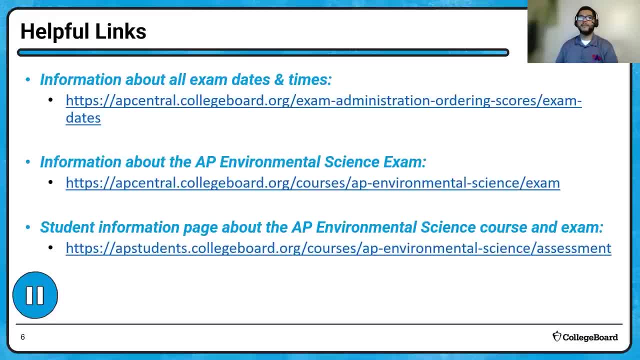 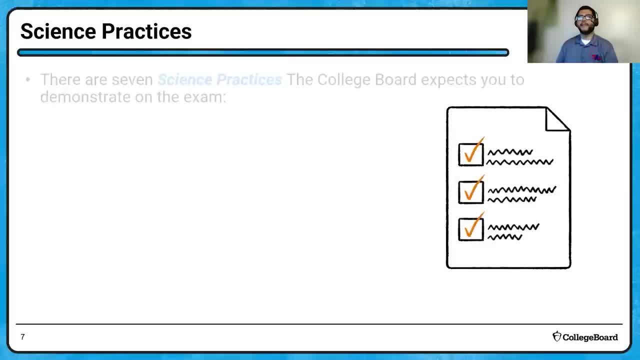 So if you want to pause that and take it or take a picture of these, you can do so and look at those as you need them. And then here's our science practices that we're going to revisit today. Remember, we do have to demonstrate concepts, visuals, text analysis, scientific experiments, data analysis. 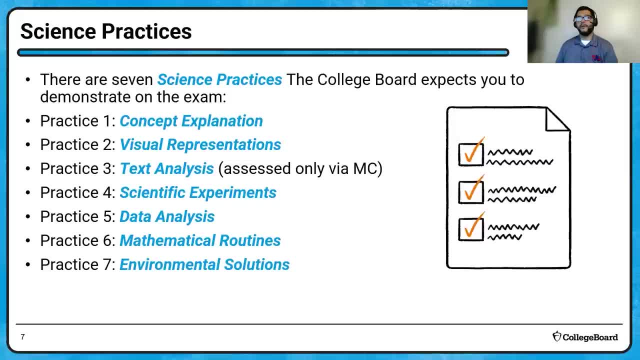 math routines and, of course, solutions. Now, don't forget that we will only be looking at text analysis in the multiple choice, but any of these skills can be looked at in any of the questions, So don't forget to be watching for those. 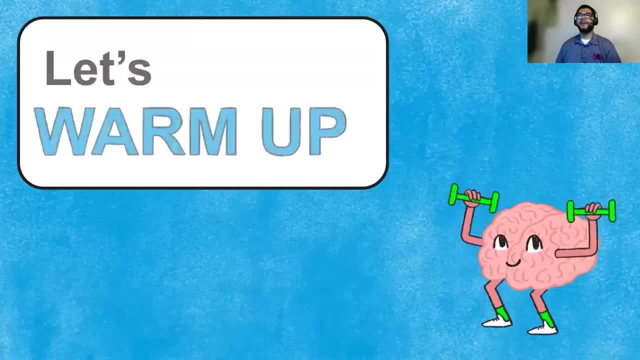 All right. So we got a lot of content to cover, So let's go through this Now. remember, we're not going to be able to cover everything in this content from these two units because they are both pretty big and pretty important. 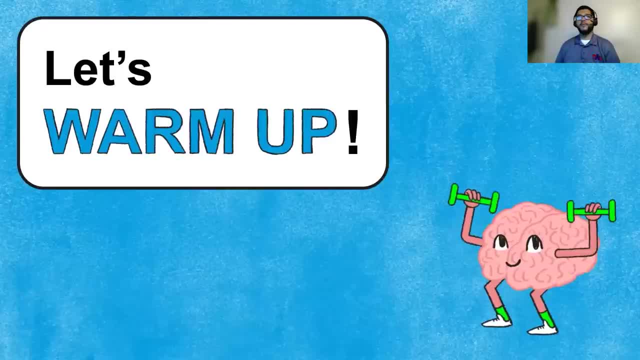 And these also tend to be students' weakest ones. So if there's gaps in this, if there's sections or topics you feel like you did not cover, we don't cover enough, well enough today, then please go back and look at those. 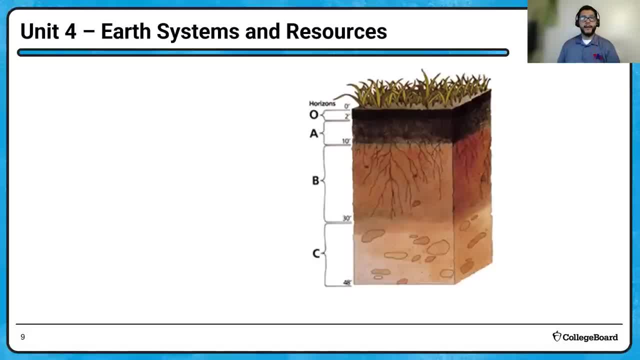 It's going to be really important. Okay, So we start here with earth systems. Now, this is a picture you should be very familiar with. This is the soil horizons, right. So soil is going to be a big deal, And don't forget sand, silt, clay. 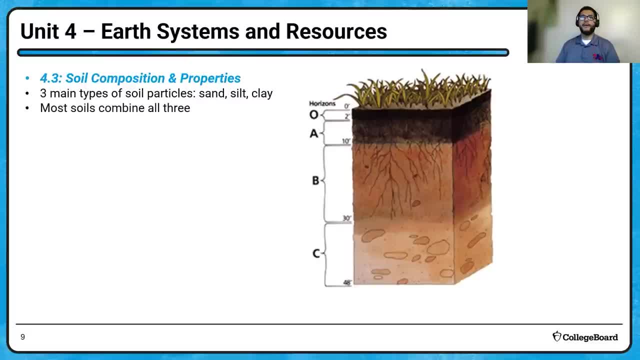 Hopefully you got a chance to do an experiment like that with your environmental teachers And you got a chance to identify the sand silt Clay in your soil And of course, it can be determined by percentages. So, knowing the percents of sand silt clay and using the soil triangle, 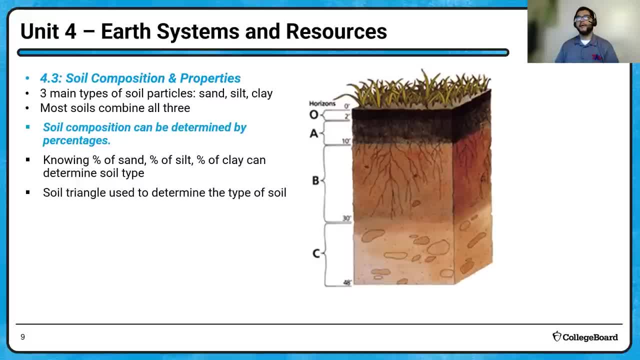 We're going to do a little bit of practice with that today and you'll get a chance to look at it And, of course, please make sure you look at as many examples as you can, but you don't have to memorize soil types. 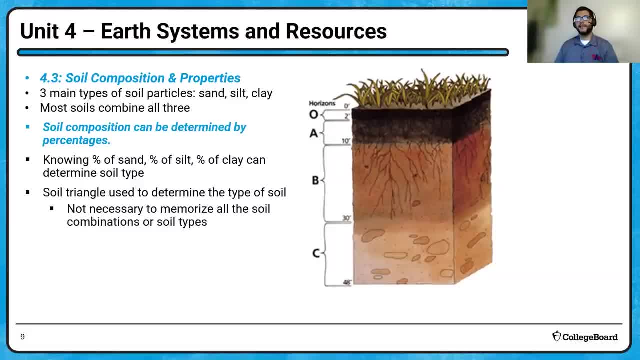 So you know. a lot of times you hear the terms clay, loam, silty, clay, silty, loamy, sand, things like that. You don't need to memorize those, You just need to know how to use the soil triangle. 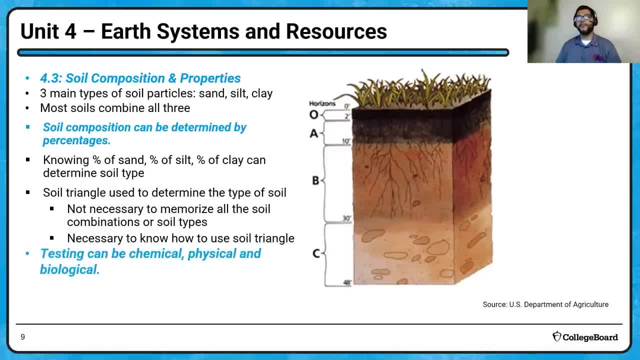 And of course the different tests that can be used- the chemical, the physical and the biological tests- to determine basically the health of soil. So be familiar with those And don't forget that organic matters at the top And then you have your top soil. 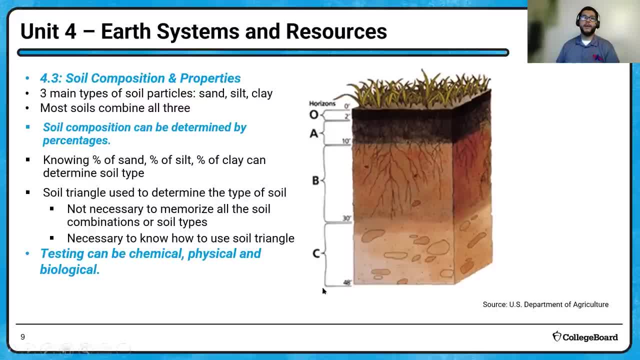 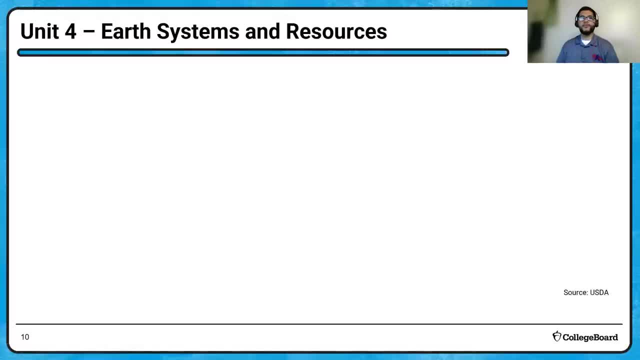 And then all the way down. sometimes you can see on the very bottom down here an extra little section called the R. That's the bedrock, And the further you go down, the more like that bedrock those soil profiles are. So here's my favorite using the soil triangle: 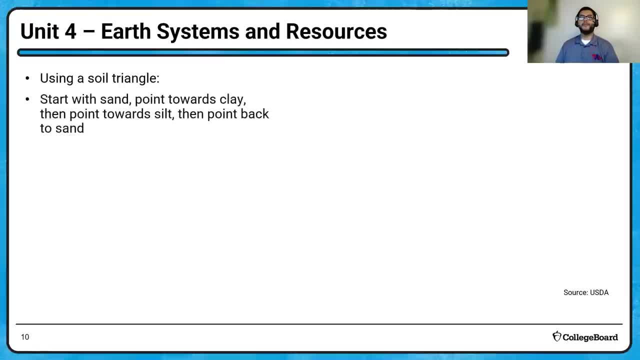 Now I'm going to show you how to use the soil triangle here, And then I'm going to show you how to use the soil triangle here, And then I'm going to show you how to use the soil triangle here. And I always say: start with sand and then point your arrows towards clay. 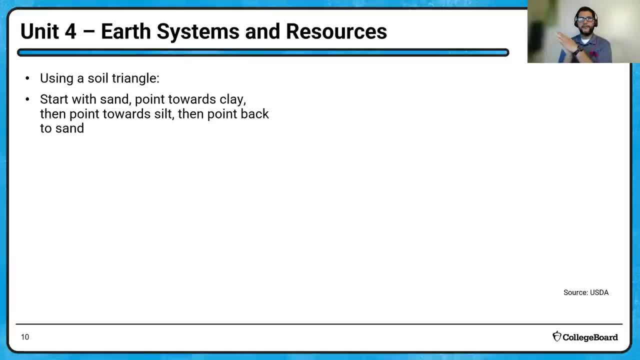 And then from clay point your arrow towards silt And then from silt point back to sand. So you're going to see how that works right now, And so if we have a type of soil- excuse me, sorry, That's 35% sand, 30% clay and 35% silt. 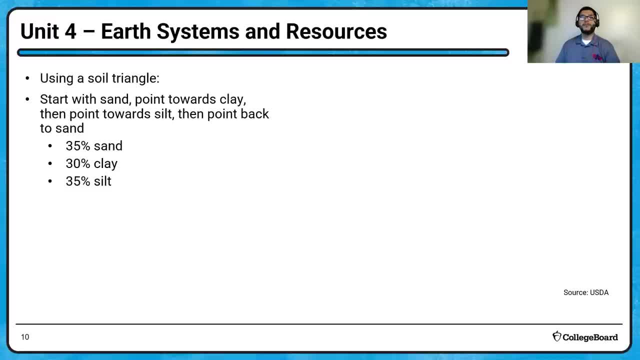 We're going to look at how to use the soil triangle here. Now, why is all this important? before we even do this, We have to understand that certain things can get into the water. Number one is it can get into the soil. Number one is water. 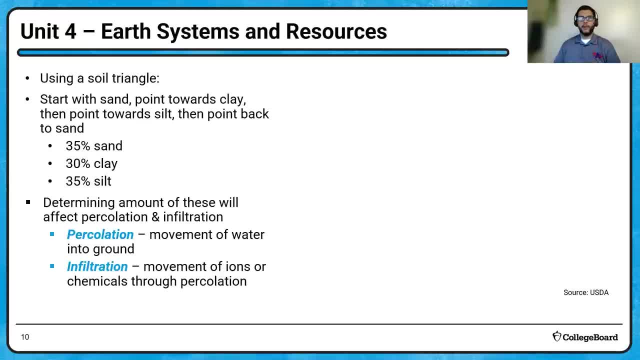 That's percolation, That's the trickling down of water into your soil profile, And then with that sometimes ions can travel down and that's infiltration. Infiltration can be good in the case of nutrients or it can be bad in the case of pollutants, but that's what that means. 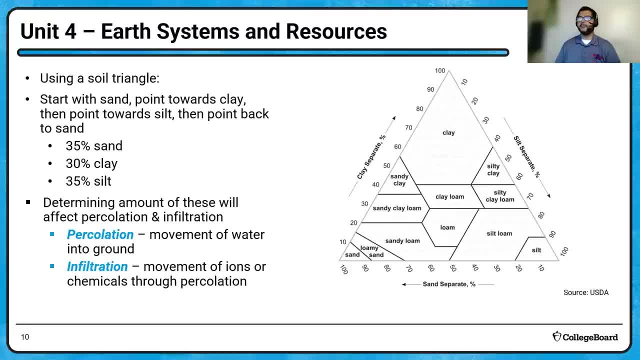 So here's our triangle. Now, let's say it's 35% sand. So what we're going to do is we're going to draw a line at 35%, And that's going to put us right here. right, And, like I said, from here we will then move and start at the clay side and look at 30%. 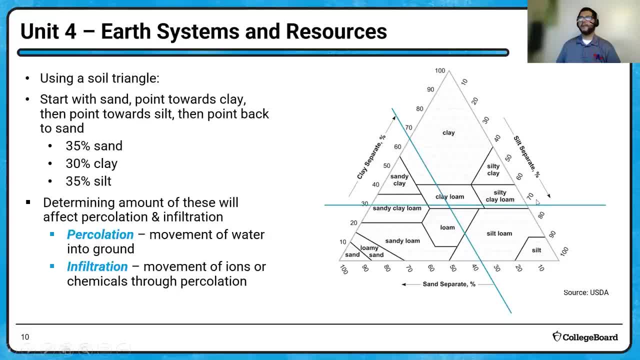 So the clay side line is going to be a straight line, always Okay. So sand is going to be angled towards clay, Clay is going to be angled towards silt And then silt is going to be at 35, right around here, angled back towards sand. 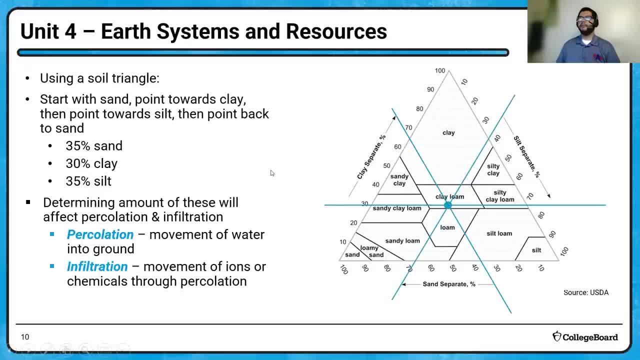 And so we see, right here, this ends up being right there at clay loam. Okay, So that's as easy as it gets. We'll go through that in one of the multiple choice examples, but be familiar with it. Either they will ask you to use the percentages and find the point. 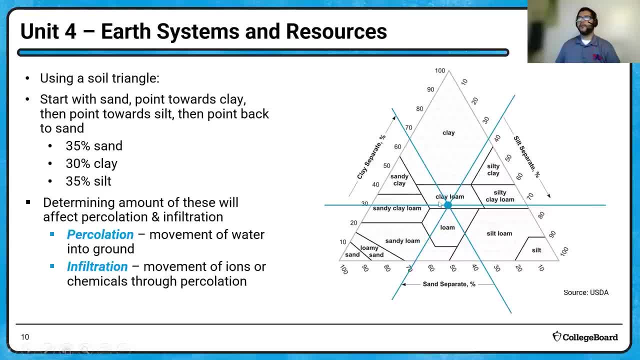 or they'll ask you to find the point and then what are the percentages? And also another way this has been asked before is if they have a point right up here, you know, where it's very high in clay, where it's like 75% clay. 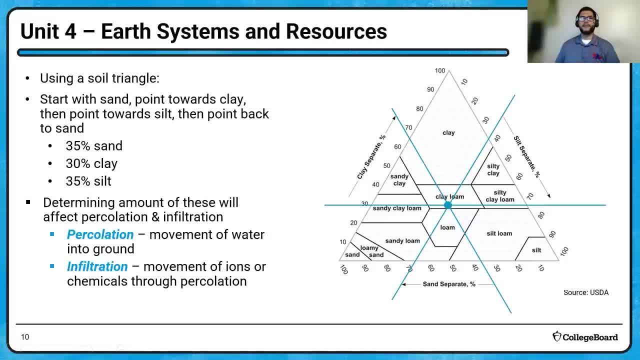 they'll say: what's this going to do about water holding capacity? Is it going to hold more or less? And if it's a lot of clay, it's going to hold a lot more because those particles are very tiny. Okay, All right. 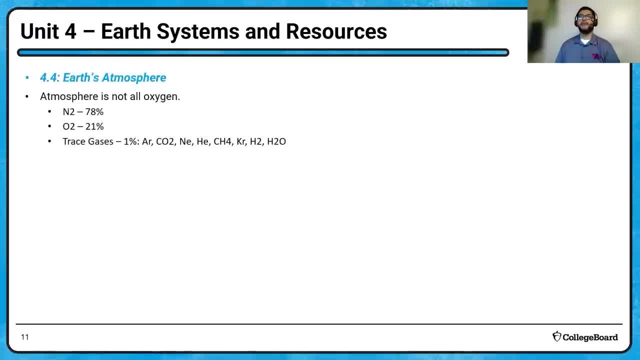 And then we get to the atmosphere, right. So we move up a little bit. and don't forget, our atmosphere is made out of nitrogen, right? 78% with 21% oxygen and then 1% of trace gases. Now, the thing to remember is that the troposphere is going to be the 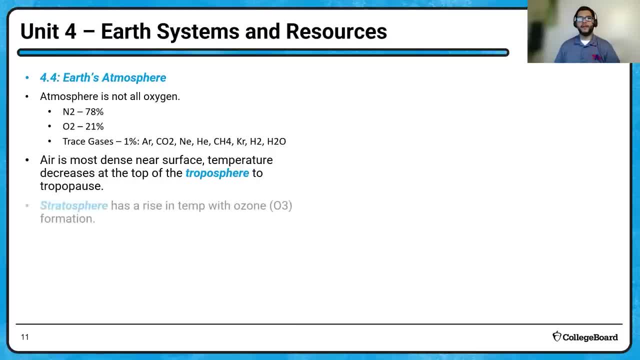 one of the two important layers, not to say that the other layers are not important to the earth, but the typical questions you get for environmental science are either about, you know, troposphere or stratosphere. okay, And then of course, we do have some changes in the temperature. 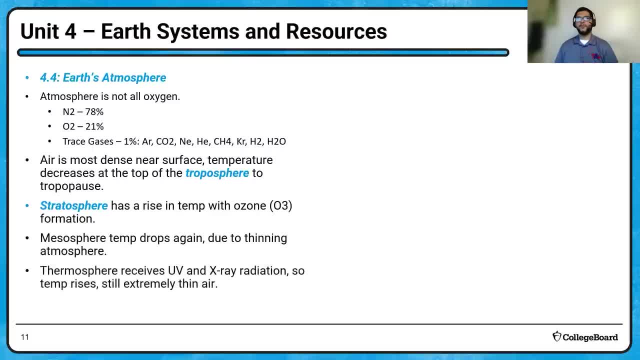 Now, the troposphere is where all the weather occurs and the stratosphere is where the ozone actually is. That's the UV-protecting substance that's up there. So you know, the thermosphere of course gets a lot of UV and X-ray radiation. 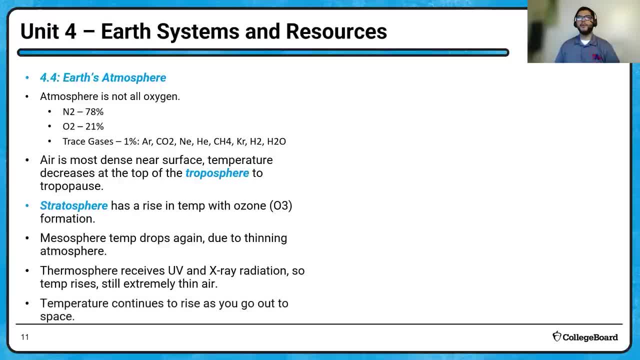 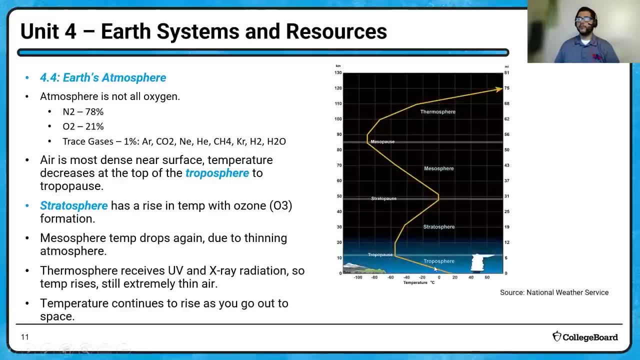 And so the temperature rises and it's extremely thin. So most of the particles of the atmosphere are down where we are okay. So if you take a look right there, we're down here in the troposphere. This is where the weather is occurring. 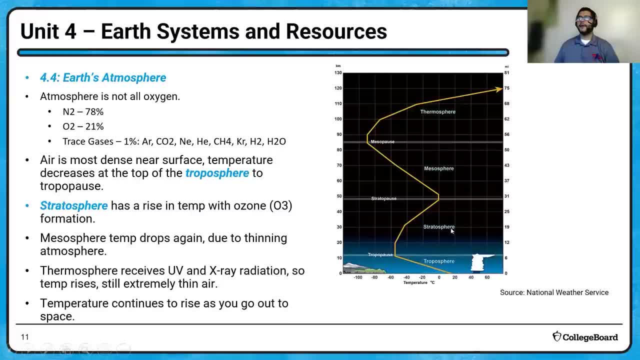 This is where the majority of particles are, And then again the stratosphere is important because that's where the ozone layer is. So not to say they won't ask a question about these other layers, It's just that the bulk of them will probably be concentrated down here. 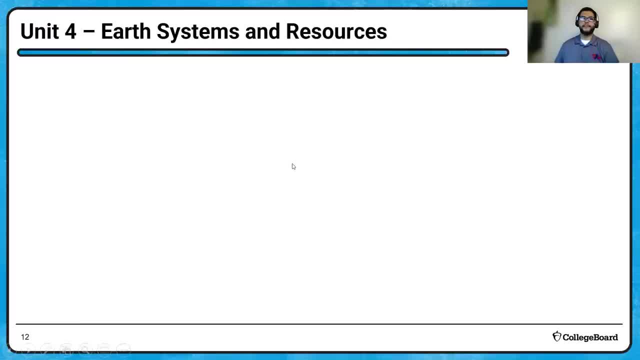 So some advice there, Okay. Then we talk about global wind patterns. So the earth has an atmosphere held to it by gravity And of course the earth is circulating, So this ends up causing, you know, the atmosphere to be more concentrated. 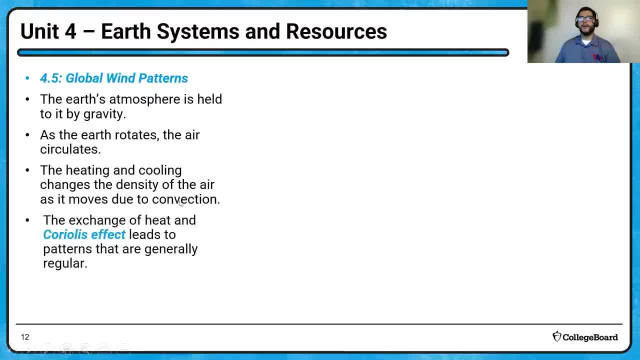 So this ends up causing the atmosphere to be more concentrated. So this ends up causing the atmosphere to be more concentrated And this in a way leads to heating and cooling of that air, and this process we call convection. okay, And that Coriolis effect leads to these patterns that are pretty regular. 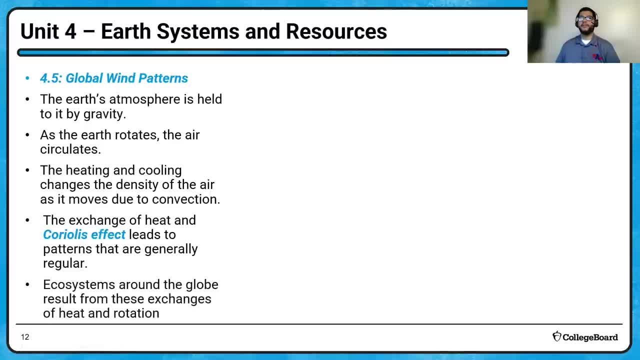 And ecosystems around the world look certain ways. So when you see this, don't forget. you know we see deserts at the same lines of latitude, those lines across right. I always tell my kids my jokes and I say: you know, latitude is fatitude. 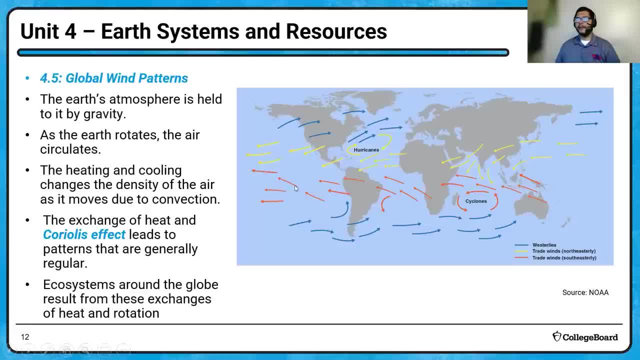 It goes wider right And so if you look at it right here, You know these wind patterns are pretty much general all the time. So you see right here that everything the biomes on this line right here tend to be pretty, very similar The biomes at 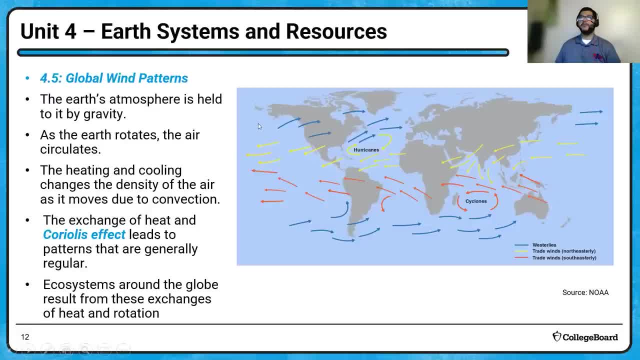 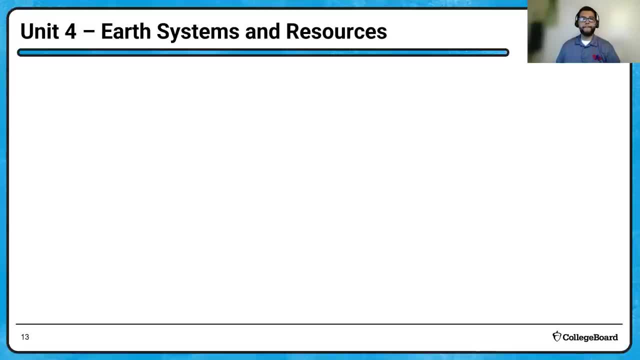 this line over here tend to be very similar as well. So please make sure you review the biomes of the earth from unit one so you can see where those go right. And then, of course, we get to the solar radiation and the seasons right. So the first key term that a lot of students don't remember. 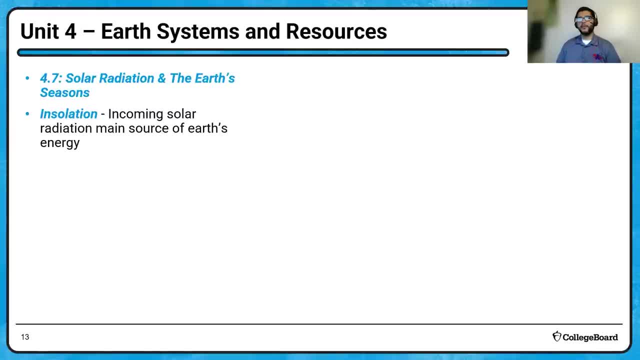 is something called insulation, And that's the idea that the solar radiation is the main source. So you may hear that term when you get questions like this, So don't be shocked. It's just, you know. energy from the sun, okay, And of course the tilt of the earth is the reason for the season. 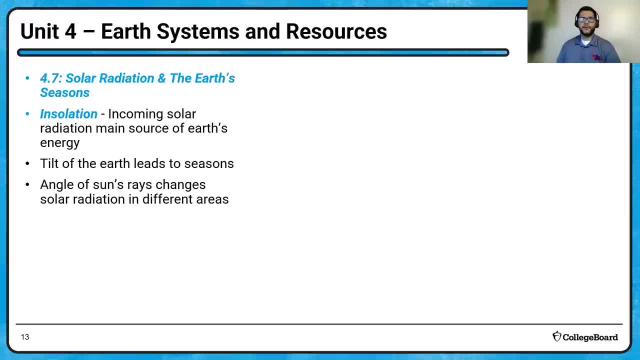 right And the angle of the sun's rays. that's what causes that different amount of solar radiation everywhere with that tilt. So you end up with certain parts that get a lot of- you know- sun and a lot of heat And other parts that get a lot of heat right, So you end up with a lot of heat. 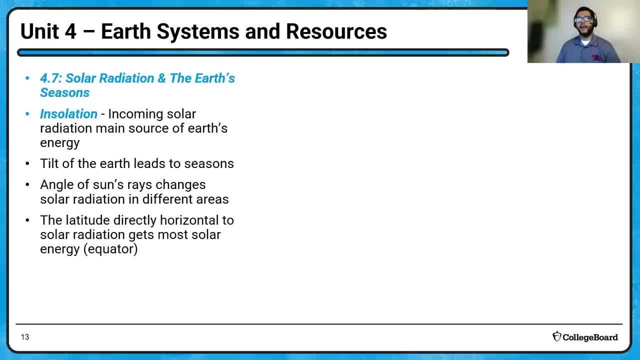 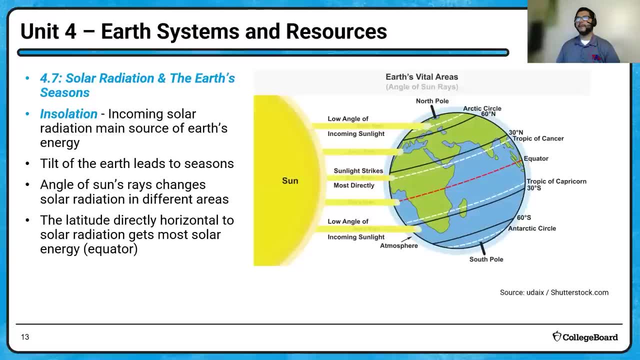 get more of a seasonal type area right, And so that line of latitude is directly important. So if you look at the one that is our equator line, that's the one that gets the most sun. So right here our equator gets the most sun the most part of the year And it's right in between the 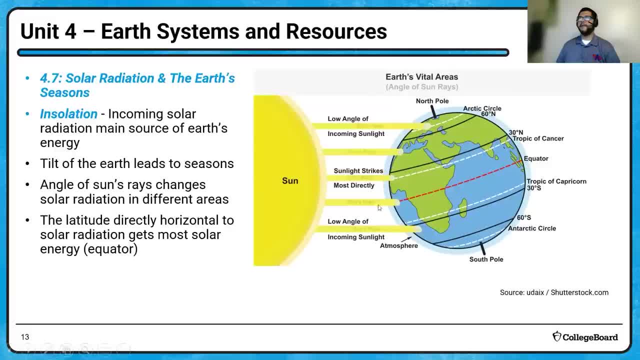 Tropic of Cancer and Capricorn right, 30 north, 30 south. That's where it ends up being very, very sunny all the time, And then, of course, in this picture, when you see the sunlight's rays coming. 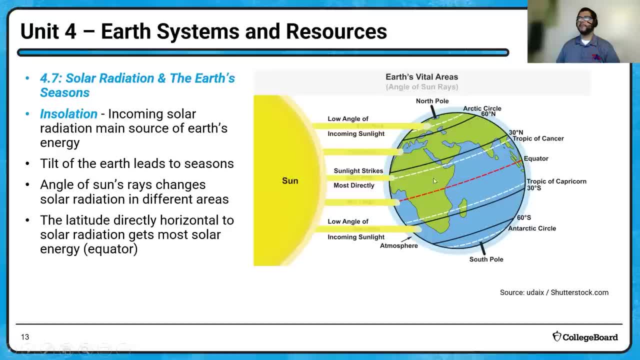 up on the north it's the most sunny part of the year, And so that's where it ends up being very northern hemisphere more. that's going to be their spring and summer And that's going to be the southern hemispheres winter, And then, if we were to flip this right and the bottom, we're. 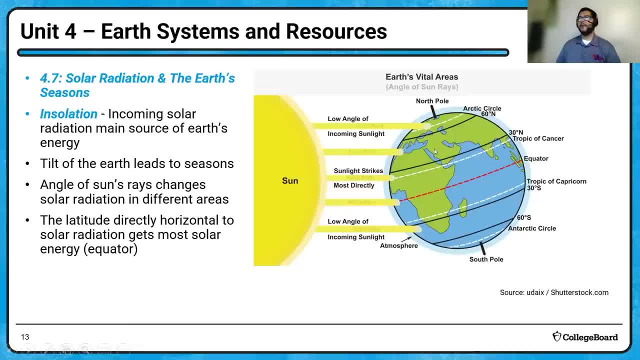 getting more sun at that time, that would be their summer, while the north is having their winter, Okay, And so that's an important thing to remember, And this, of course, plays a role, along with that movement of wind to your biomes and their lines of latitude. So that's going to be between that. 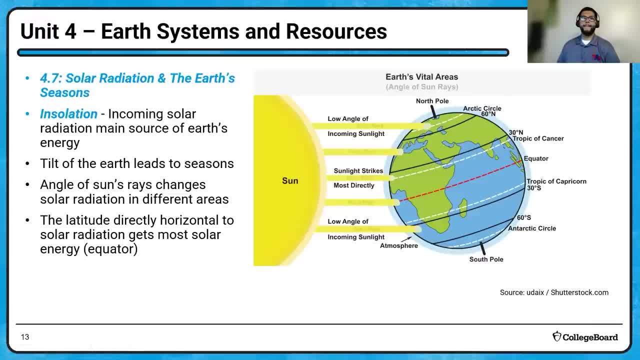 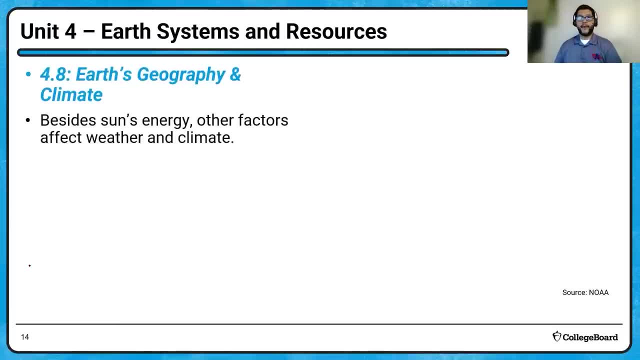 and the wind patterns. That's going to be a really common thing, Okay, Okay, And so, moving on, we're going to be looking at geography and climate. So, besides the sun's energy, that is a big factor, right, obviously, But there are other factors that can affect weather and climate, And the two big ones: 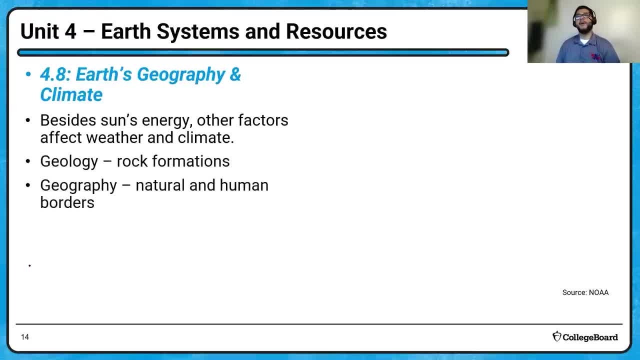 are geology and geography, So know the difference between those. Geology is going to be your rock formations like a mountain or a valley, Whereas geography is going to be a natural or human border, For example, the edge of a city versus the edge of a forest. That's going to be a natural or 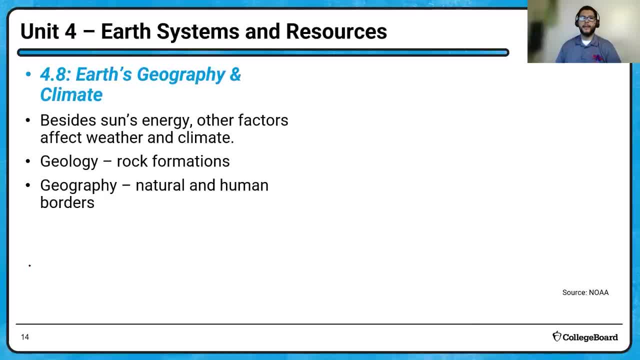 it's going to be a change in geography. right, That can be a human-caused one, And so this is most commonly seen for geology in the form of the rain shadow effect. This is going to be where this region of land becomes drier because the wind comes in from one side, from the coast, and that's 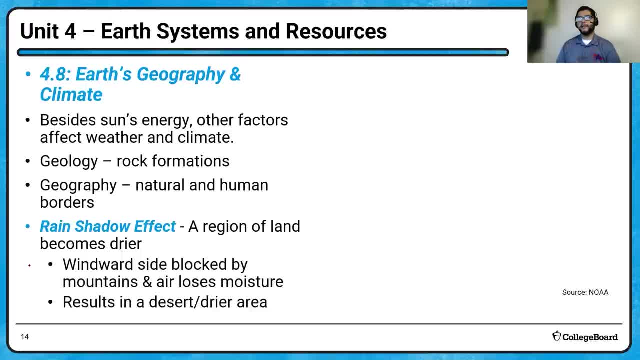 the windward side, and it's blocked by mountains on the other side, to what we call the leeward side, And that ends up drying out a bunch of the air as it goes, And so what that does is it ends up creating a 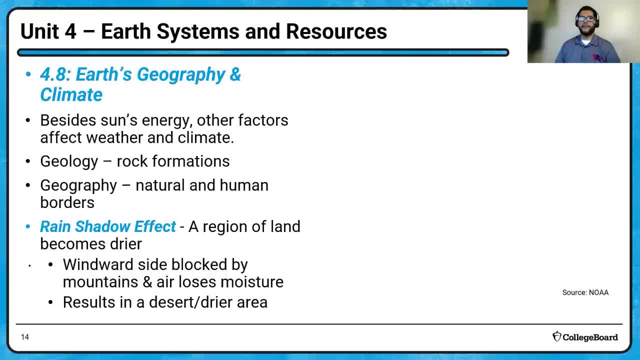 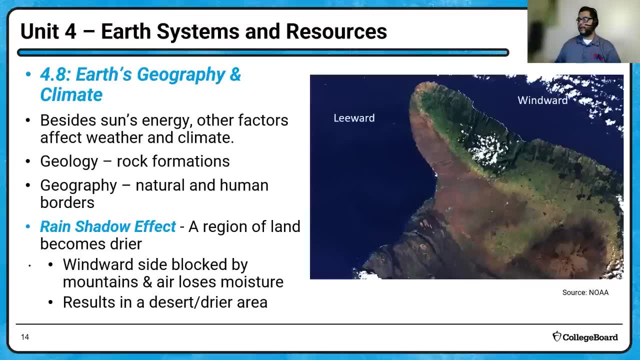 It ends up creating a desert-like effect. So if we take a look here, right, This is the big island. I believe in Hawaii, And so what happens here is the wind comes in from the windward side and it blows to the coasts right, And it has a lot of moisture from the ocean, So it's nice and green. 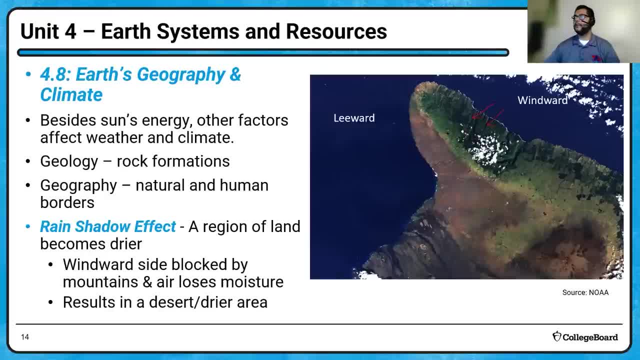 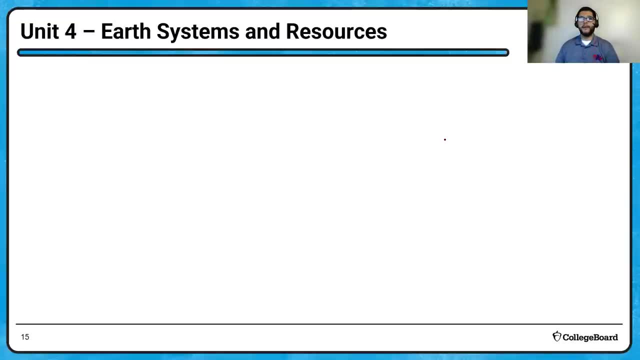 and lush on this side, Whereas over here, your leeward side, the air moves up and it dries off and this ends up becoming a desert-like area. So you end up with that dry, desert, lack of moisture air right, And so, from here, right. other concepts to finish up Unit 4 with are, of course, El Niño and La Niña. 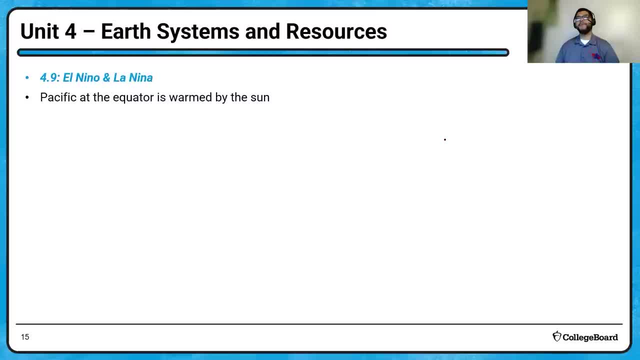 This is a really important one. So some background about this. It's all about the Pacific. They always ask, sometimes simple questions about what ocean does this occur in? Well, it's a periodic area where the part of the Pacific Ocean gets warmer than usual. We call it the El Niño Southern. 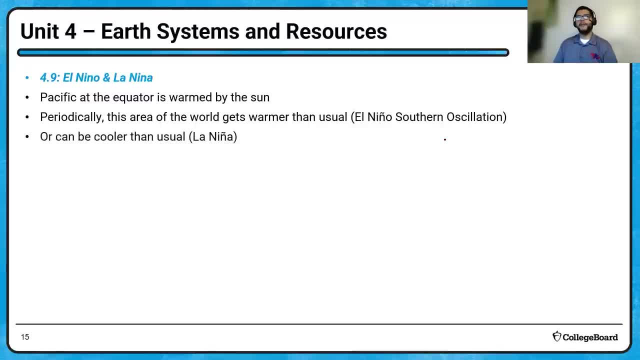 Oscillation or an ENSO right, And so the La Niña is where it's cooler than usual. So it's basically: El Niño is a warming effect and La Niña is going to be an effect where it's an extreme normal right, So it's cooler. 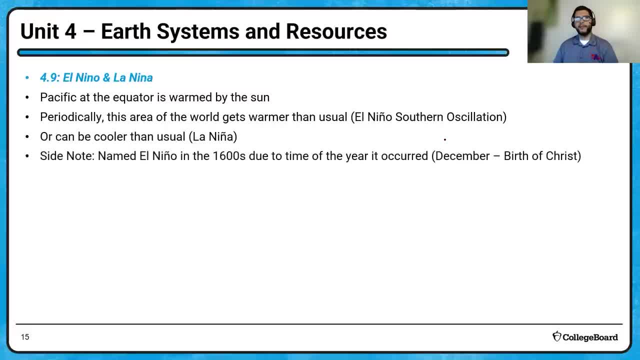 And so it was just a side note here. I like my history a little bit. El Niño was named in the 1600s because of the time that it occurred. It was usually in December, which is the birth of Christ time, So that's where it gets the name. 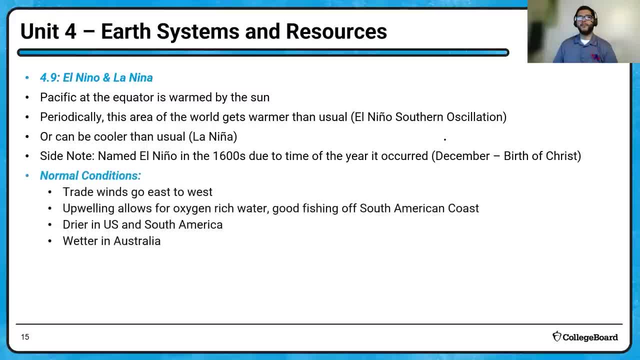 And, of course, normal conditions. Here's what you get, right: The trade winds are moving from east to west on a map, and you'll see that in a moment- and then upwelling, which is the water moving up, allows for oxygen, rich water and nutrients to come up to the surface and you get really good fishing off the. 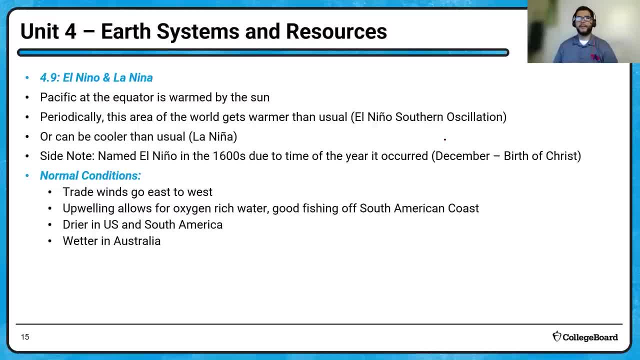 south american coast right, mainly anchovies- is going to be a big- uh, a big fish that we get out of there, and then we get drier us air in south america and then, of course, it gets wetter in australia, so they get more storms. now in la nina, right, that's going to be an extreme version of the. 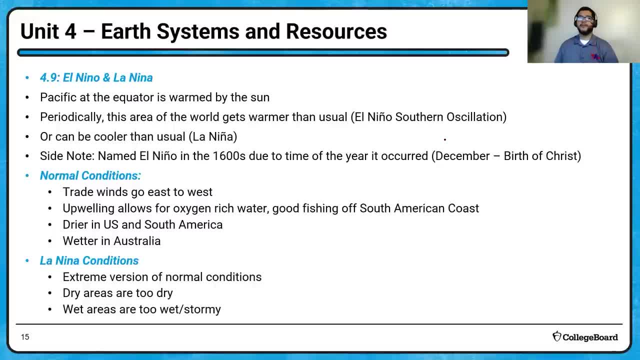 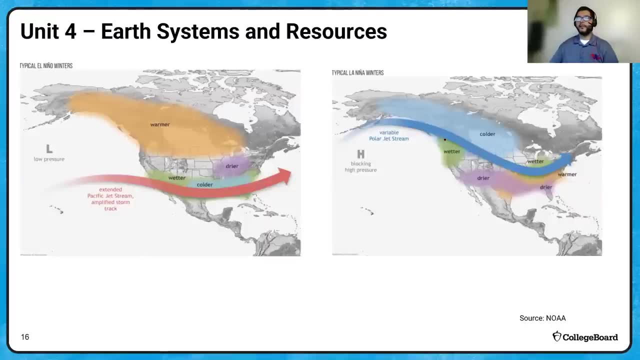 normal conditions. basically, the dry areas in the us become too dry and get drought in south america, and the wet areas get, uh, too wet and too stormy, right, um? and so here's kind of an? um a visualization of what these look like. right, if you take a look um the typical el nino winter, you end up with this: 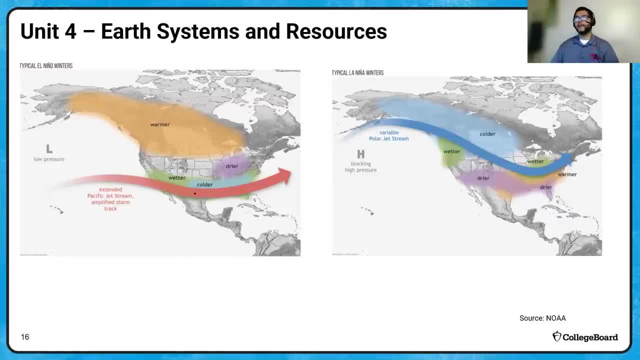 heat, jet stream amplified going through and so so, so sometimes we end up with more storms, um, but for the most part it ends up with a lot of drought, whereas a la nina winter that's where it ends up being tons of drought because that jet stream is. 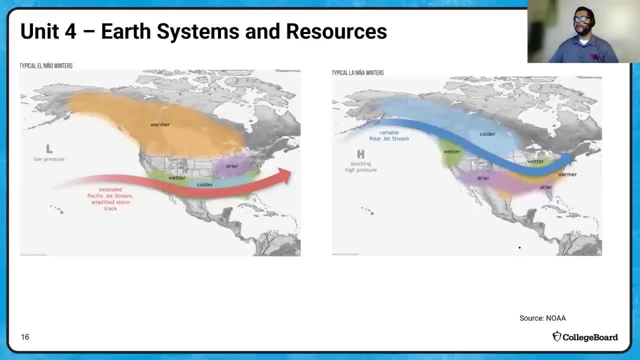 moved, because over here, down on this portion of the pacific, right, if you look over here in an el nino year, this warm spot is right here and there's no more nutrients. and, uh, in a la nina, that warm spot's not here. it's actually over here closer to australia, okay, and 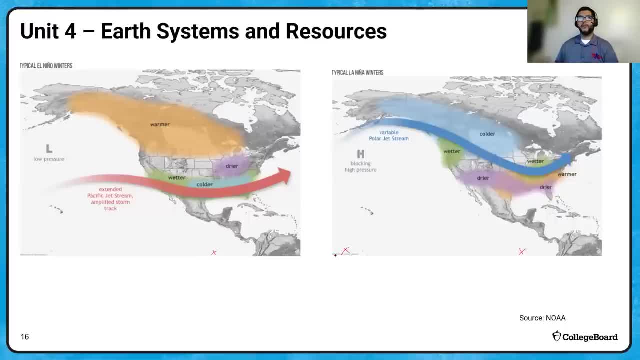 so that's a really common thing, so make sure you're familiar with it. if you need more help with it, uh, make sure to look at, uh, la nina and el nino. okay, and that's unit four. so let's look at unit five now. um, and of course, we begin with tragedy of the commons. that's probably the most important thing. 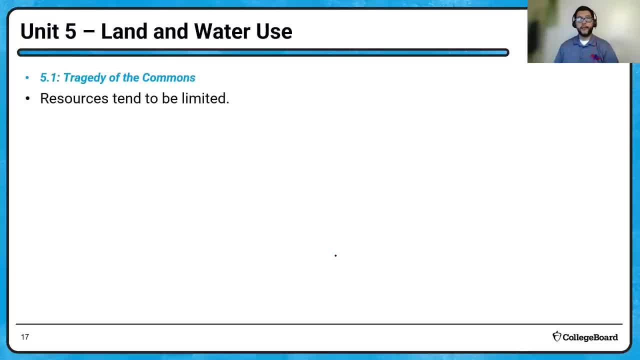 that's about resources being limited. right, hopefully you did a lab or an activity with your teacher. uh, this year with tragedy of the commons. if not a brief summary, the idea is that we tend to use limited resources pretty frequently and we tend to use limited resources pretty. 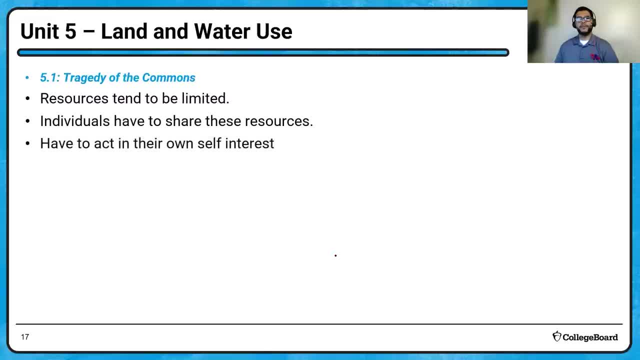 fast and the catch is we had we act in our own self-interest, so it's kind of an economics concept. it's not so much a science concept, it's an economics one and the idea is that, you know, we tend to sacrifice the common good for our own self-interest. you know we tend to be a little. 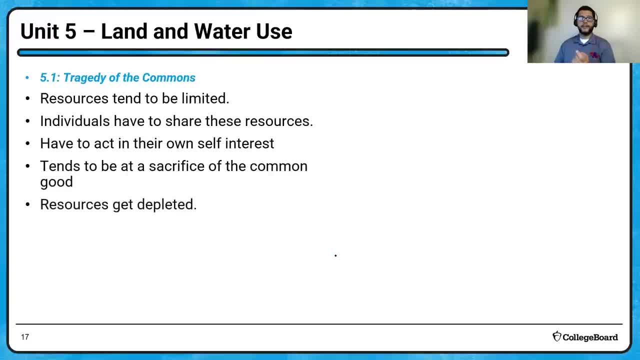 selfish, and that happens and, of course, our resources get depleted. so real life examples of this are going to be: you're over grazing in pastures. you're over fishing the oceans like passenger pigeons. those were hunted because there were so many and abundant, uh, in number. 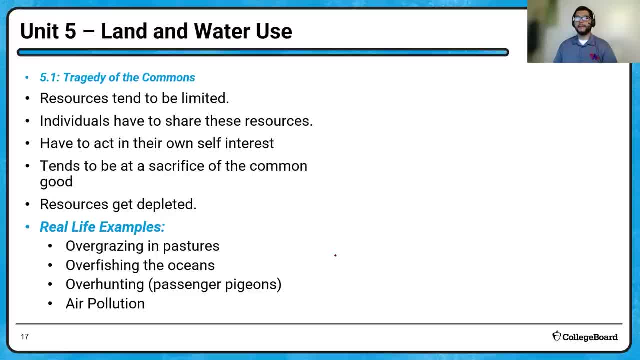 and then, of course, air pollution. that's going to be a type where we tend to have. you know, no one owns the atmosphere, so we use it as we need to and we don't pay much attention to it, so it ends up getting polluted, and that's one thing i would say is some studies have shown that when you 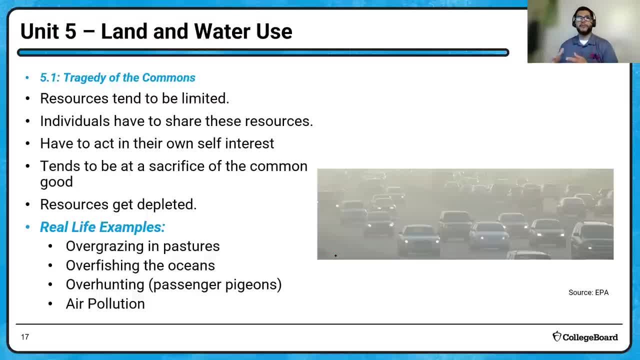 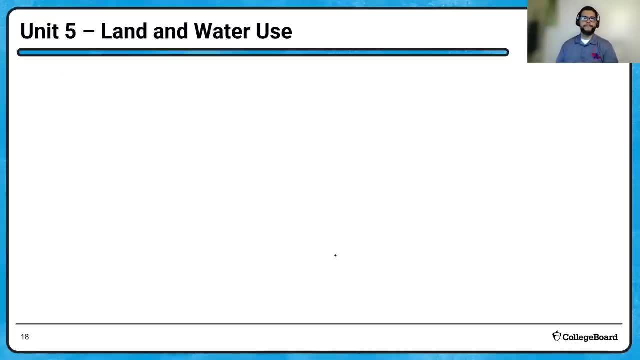 privatize things. that tends to help save the resources more. um, but you know that's up in the air as well. yeah, so it's just a matter of whether or not we can recognize a tragedy of the common and figure out how to solve the problem. okay, and so from here we get to clear cutting right. um, this is going to be a way. 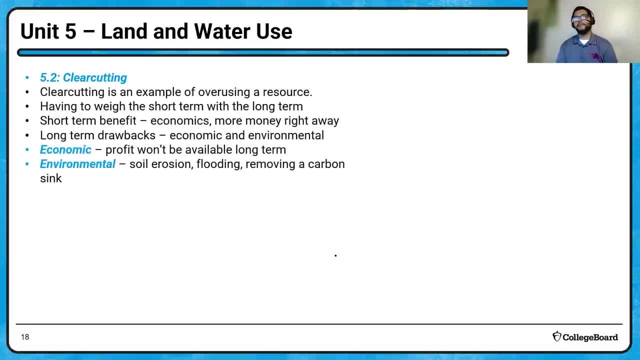 that we there's benefits to it and there's um downsides. so that's one thing i do want to point out. um is: don't forget that the ap environmental exam is going to ask you for the positives of certain things. so it's not a we're not trying to turn you into green tree huggers. we're trying 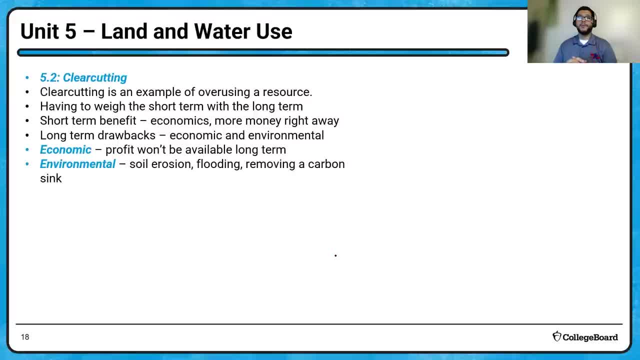 to teach you the science of it. and so they may ask you what's a, what's a economic benefit of clear cutting? well, there's profit, but it won't be available long term. so you can say: there's short-term profit, right. and of course there's many environmental problems with clear cutting. 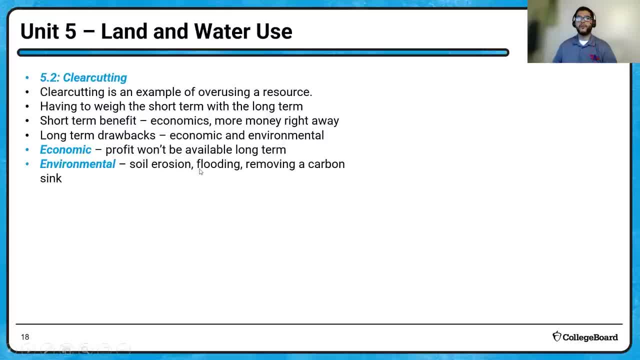 is that you're going to end up with erosion, flooding, and then, of course, you've removed a carbon sink, you've removed trees that could store carbon for us, so that's definitely something that. that's a good example of how you can get positives and negatives, and then, of course, the green revolution itself is rife with those it's going to have, uh, tons of. 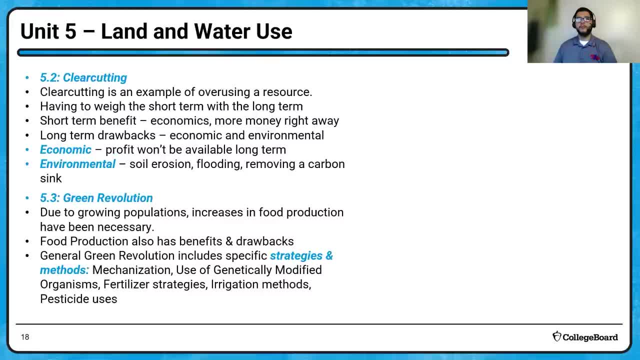 positives and negatives, and so because our population grew- remember we talked a little bit about this with malthus and how he predicted there would be, you know, famine, uh stress on the economy, or you know uh war and things like that disease. well, green revolution has kind of staved. 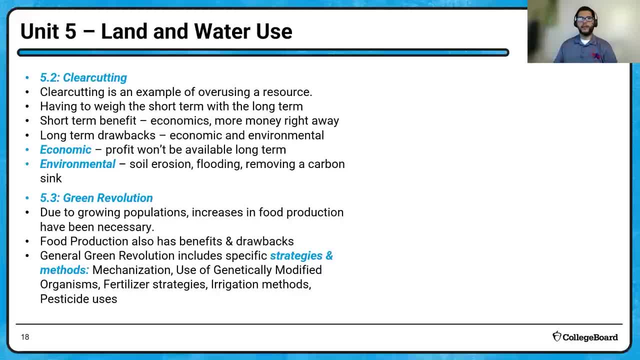 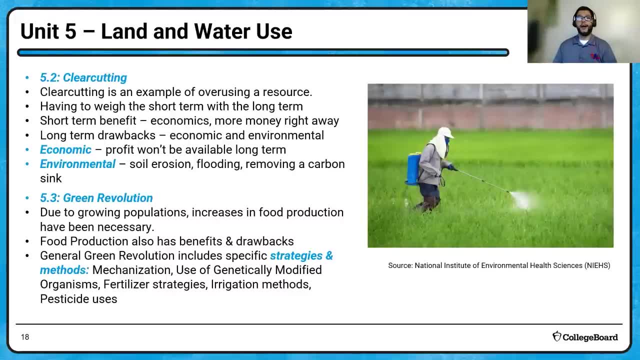 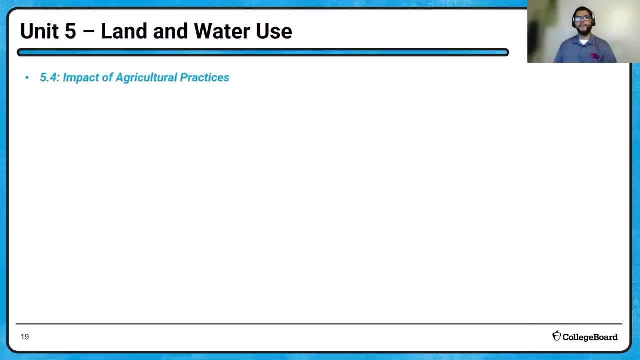 that off, um. we've had mechanization organism, genetically modified organisms, fertilizers, irrigation, pesticide use. while those don't seem all positive for the environment, they have been positive for our population and we've allowed to, we're allowed to continue growing more food, bigger food, um, so that we can have that available to us, okay. and then, of course, we get our agricultural. 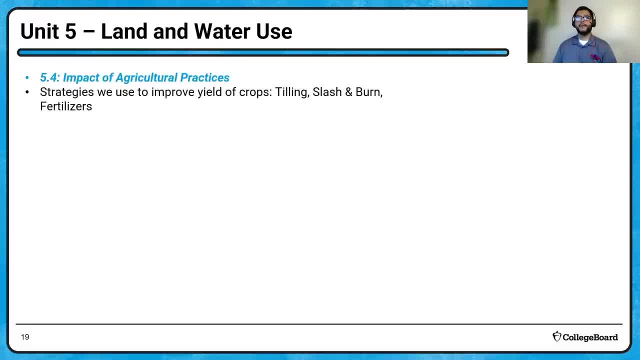 practices. there is an impact, right, of course we get uh tilling with slash and burn and of course fertilizers, so tillings um allowed to loosen up soil, put in seeds um and aerate the growing or whatever the receives as well, and help suppress weeds uh. but of course there's negatives. 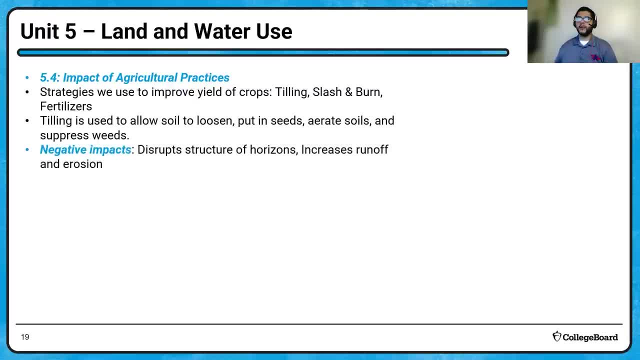 saying that it's going to disrupt the soil horizons, it's going to increase runoff and erosion um, and then it's going to end up having its own negative impacts and, of course, slash and burn is going to have a forested area or with crops in there, and it's going to return nutrients temporarily right. 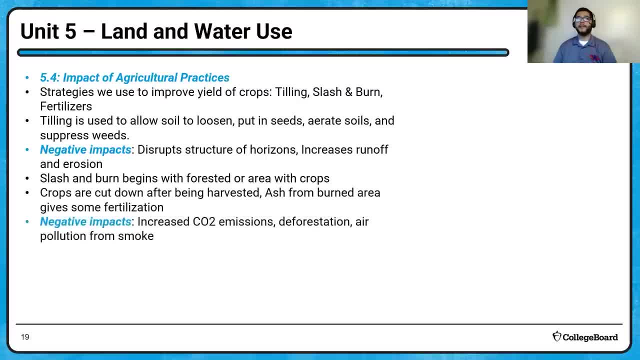 once the ash is put in there. but of course it's going to increase co2 because you've got deforestation. if that was a forested area, it'd only go up to 100% of that phosphorus which would. so that's the loveseek number one, the most popular and the most healthy. number two is the the most. 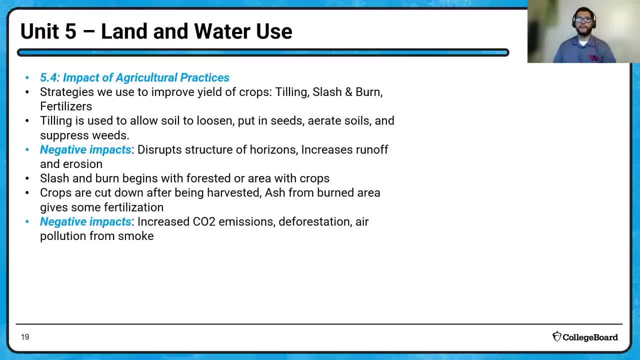 first, And of course the air pollution from the smoke. And then of course the fertilizers are important because they're made commercially And remember we talked about cycles in unit one. nitrogen and phosphorus are limiting cycles for the most part, So adding those nutrients can be. 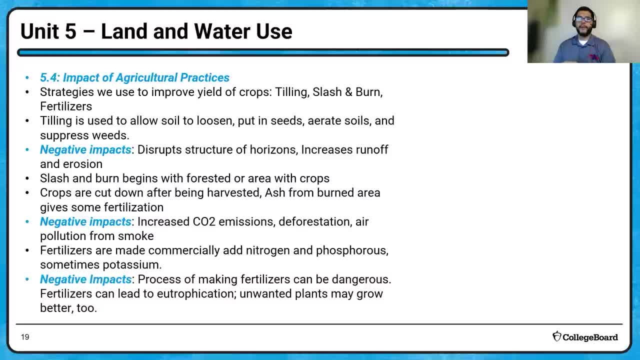 a benefit, But of course you can end up with negative impacts, where the fertilizers can cause eutrophication And of course those unwanted plants may grow better as well. So you don't have fertilizers that are unique to just one crop And of course this tilling can lead to its own. 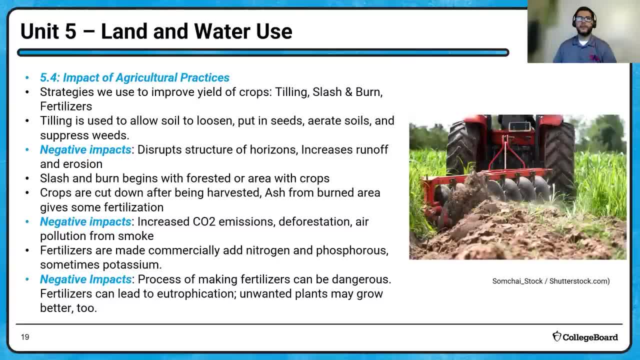 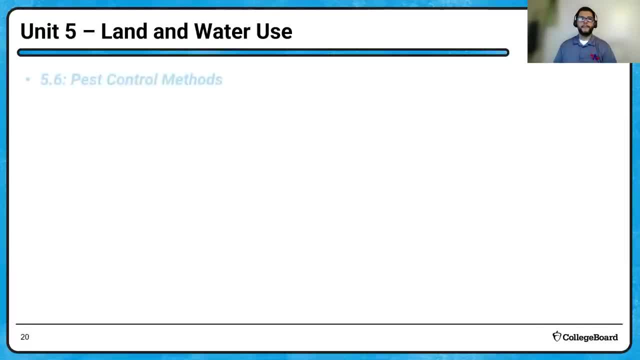 issues as well. So there's so many different things to know, but be sure you're familiar with the positives and the negatives of all these practices. Then we get into pest control. And so, of course, when we do monocropping, when we grow one crop at a time, the pests come in quickly, right? They? 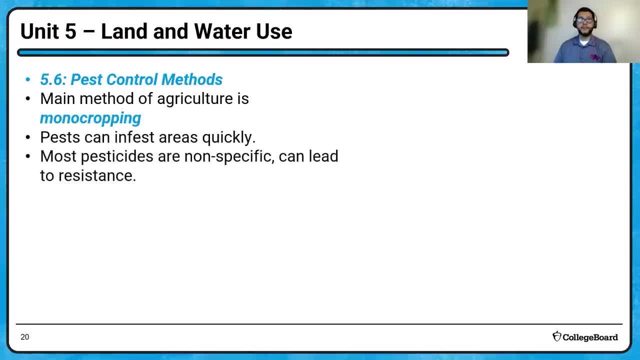 infest the area, They can be nonspecific. So that can lead to resistance as well And that means that, just like a bacteria with an antibiotic, when you introduce them to so much something to kill them, there will be eventually individuals with diversity enough to fight that. 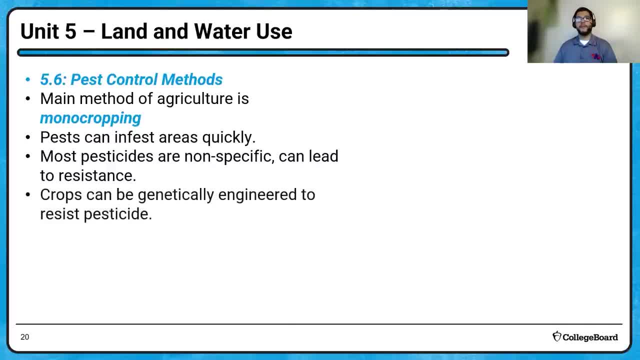 off, And so the more use of pesticides, the stronger the pest can become. And then, of course, you can genetically engineer the crop to fight off that pesticide yourself, So you can spray as much as you want. The downside I will say with this is that there is a worry that there could. 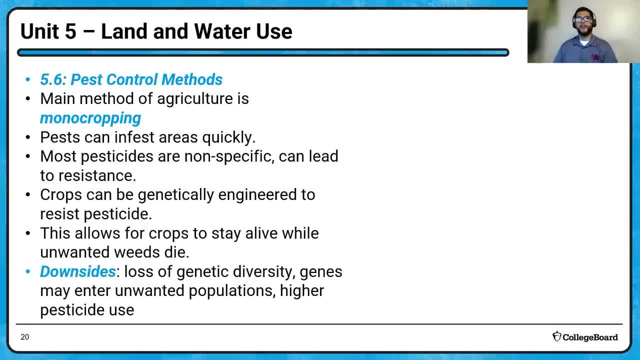 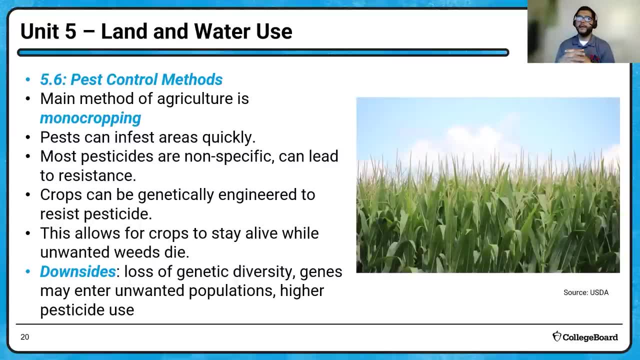 be a gene that maybe jumps into an unwanted population And, of course, the higher use of pesticides could end up leading us to get sick. right, Because this is food. It's a food crop, like corn. If that were to end up in our tissues, because those tend to be fat soluble, you'll learn. 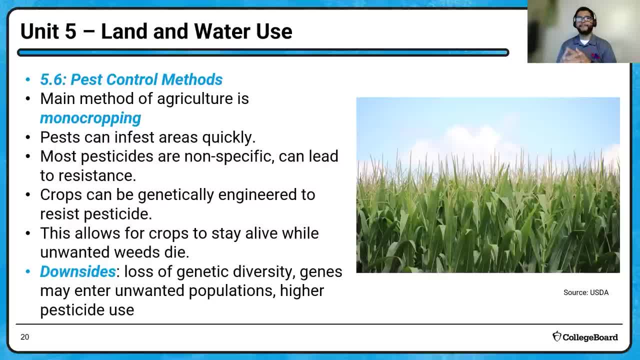 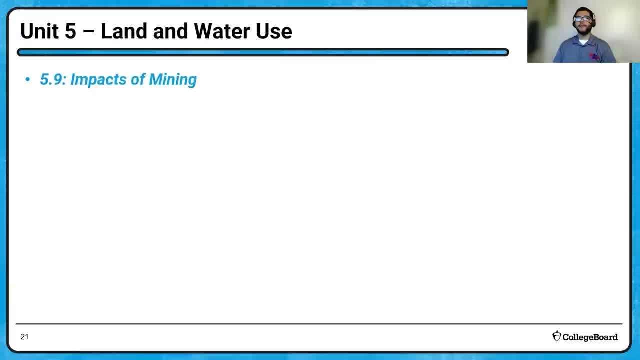 or you'll talk more about that With toxicity, but that's a that's a problem with those. Okay, And then, of course, we get to mining right. So now we're in mining And the idea is that we like to take the ore from the 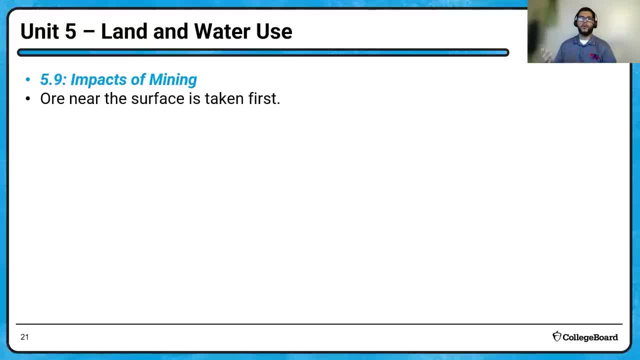 surface, that's stuff at the top right, If we're thinking coal or you know a valuable metal like gold or something. And of course we had to reach further and further down and it got more and more dangerous right And so the ore was kind of lower grade And then 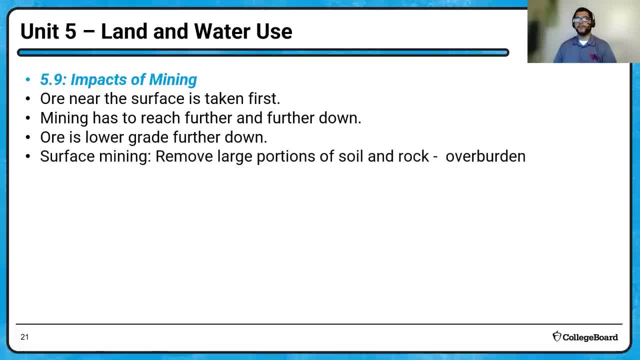 we switched from subsurface mining to surface mining right, And that of course, creates overburden, And of course, the pros to this, when it comes to coal, are many. we do get low cost energy, we do have materials for products like plastic or precious metals, But then of course, 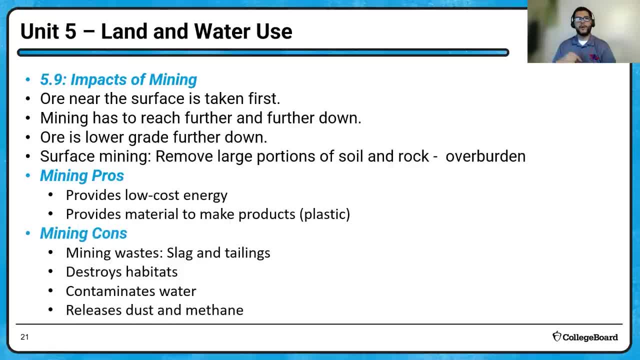 there's downsides, because we can get slag and tailings- those are going to be our waste from those mining operations. habitats can be destroyed And that's always like a good number one answer- Habitat destruction. And then of course it can contaminate the water and release dust and 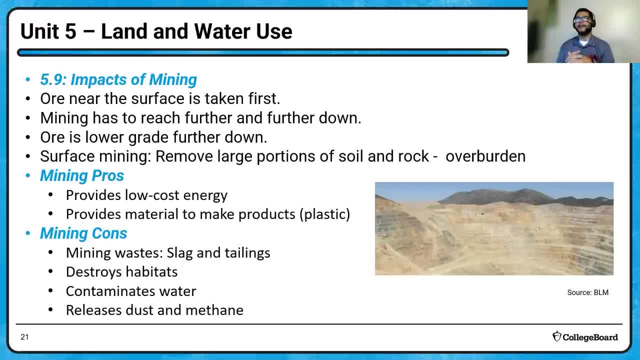 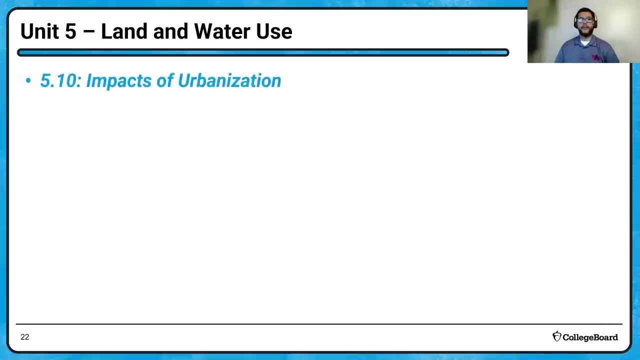 methane into the air. So it's not. they're not perfect. And of course we don't do any more subsurface mining because it's very dangerous and expensive. So most mining now is surface mining. Okay, And then of course we get to urbanization. right, We do end up having human populations. that 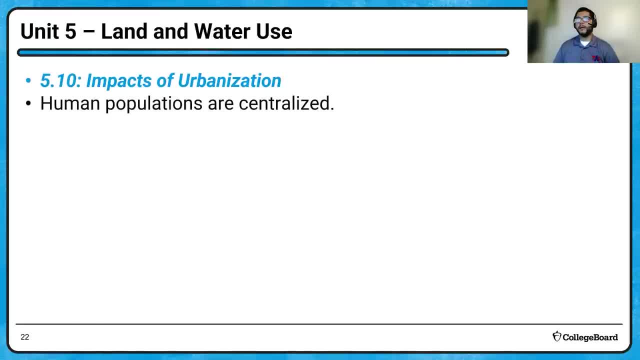 are centralized now, So we're growing around one more, you know, more and more in a central area And that can lead to several impacts, right, Of course, if you're by the coast, that saltwater intrusion, where the water comes in from the ocean. 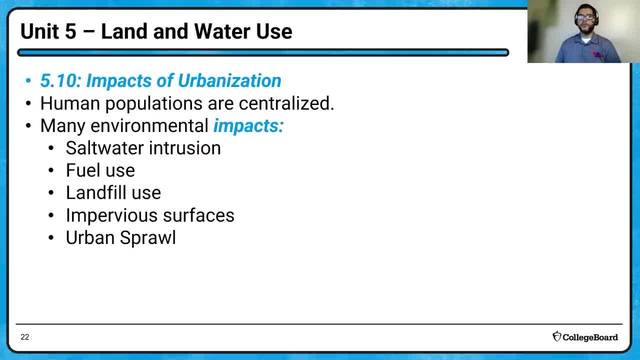 because we've used up groundwater too quickly. you can get fuel use right. Of course, landfills, impervious surface and, of course, urban sprawl. And then here's a big one with urban sprawl is you can end up with the urban heat island effect right. So basically, temperatures will. go up much higher if you take a look right now at therie of that. So we've got a lot of water and we've got a lot of landfall, So we've got a lot of landfall right. So we've got a lot of landfall. 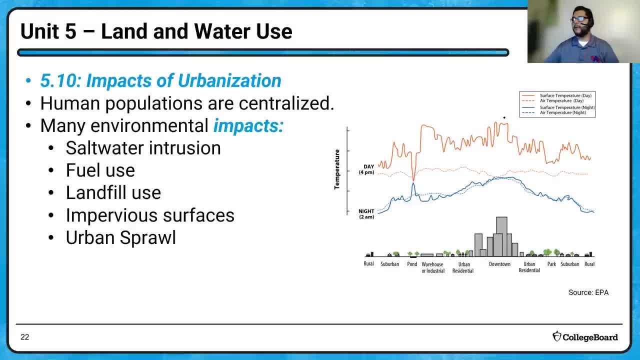 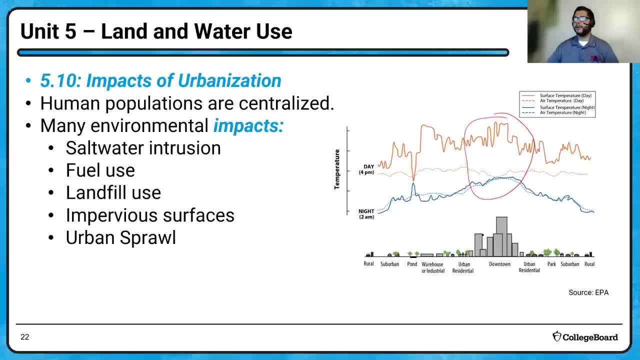 cover, and so a lot of that stuff gets absorbed by the asphalt, the parking lots, the buildings, and so you know you've got these areas where there's parks and rural areas. those tend to have the coolest temperatures, and so that's a big, important one to be considered as well. 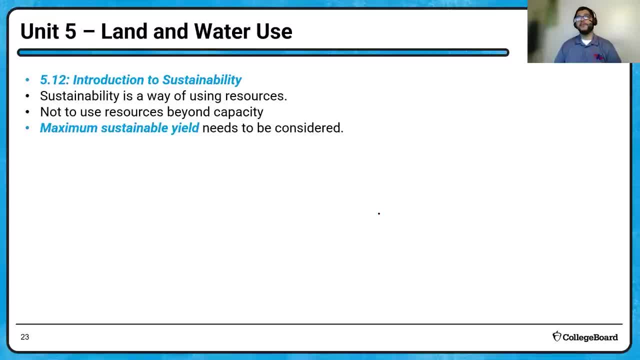 okay. and then we get to sustainability, and so for this one, this is a big, big deal, okay. sustainability is a big concept in environmental science and it's a really important one when it comes to solutions- right, because we can do a lot of these things, but we have to consider the consequences, right. that's something that, as environmental scientists, 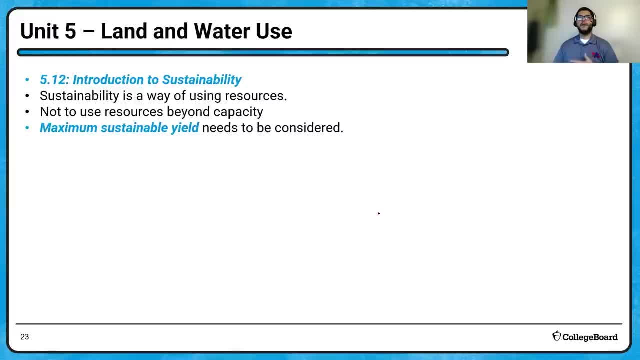 we always try to consider is: we can use resources but not use them beyond capacity and make sure we use our maximum sustainable yields right. this is the idea that we want to grow or we want to have some sort of a resource and take as much as we can without. 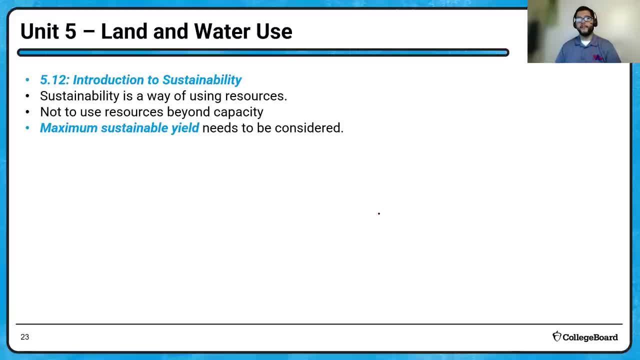 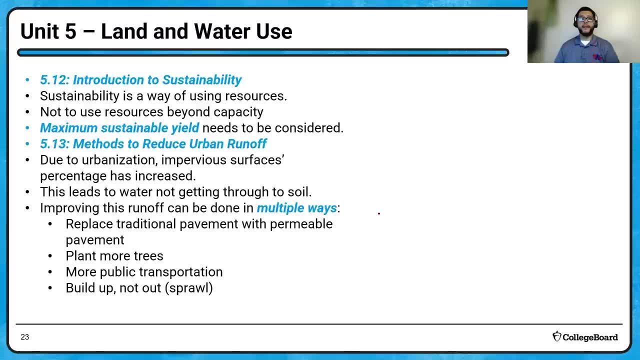 ruining it for later. this has happened before with fishing things like that, and of course, we want to find ways to reduce these things for runoff, right. so because of that urbanization we mentioned earlier, we get impervious surfaces. so when it rains, it quite literally floods, right. 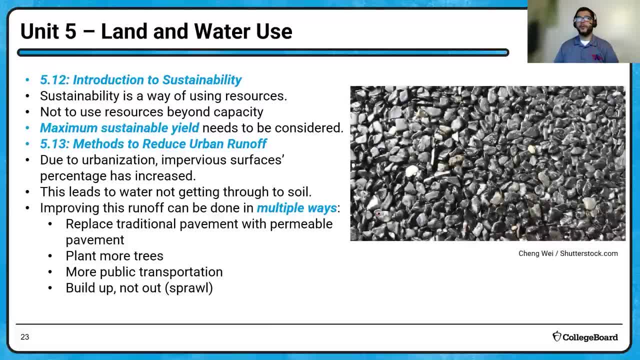 and so you can do this by several ways. if you have permeable pavement, right, if you have more loose gravel, if you have more trees, if you take more public transportation, that's going to reduce the need for parking areas and stuff like that, and so one of the new future- 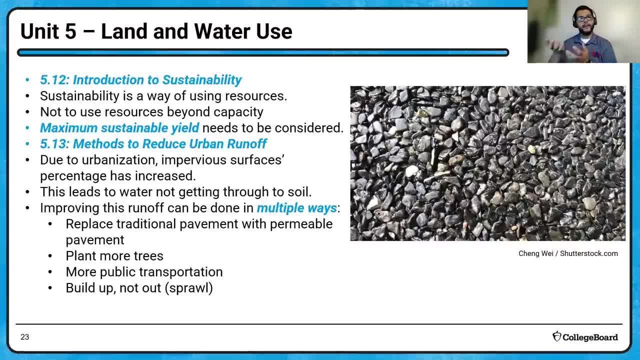 hopes that we can do is maybe if we build our places up and not out, so instead of having urban sprawl, we have urban rising instead. but that's something that takes proper planning, and if there's no planning, then that's really not an option. so it has to be something that's long-term. 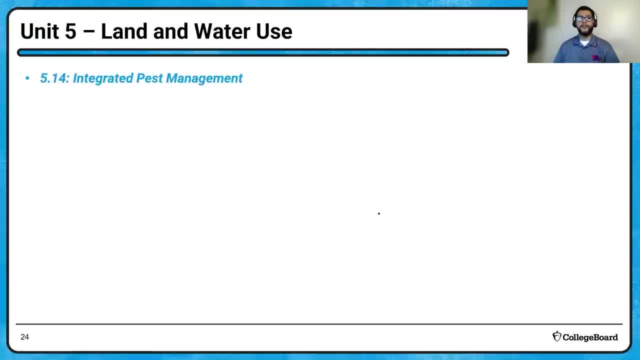 considered okay. and then, of course, we get to ipm. so, switching back over to farming, we want to make sure that we can use the same or similar methods to farming, and this does not mean never using pesticides okay. it just means trying to use pesticides as a last resort or as minimal. 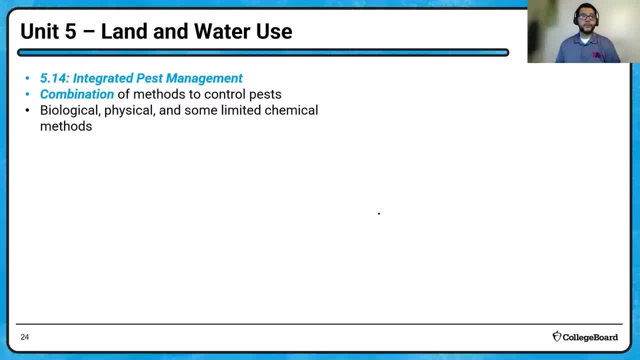 as possible. so you can use biological control, physical controls and then, of course, if it gets bad, or if you have just a few more you have to try to get rid of, then you can use pesticides. so the best part is that you can use pesticides and you can use pesticides and you can use pesticides. 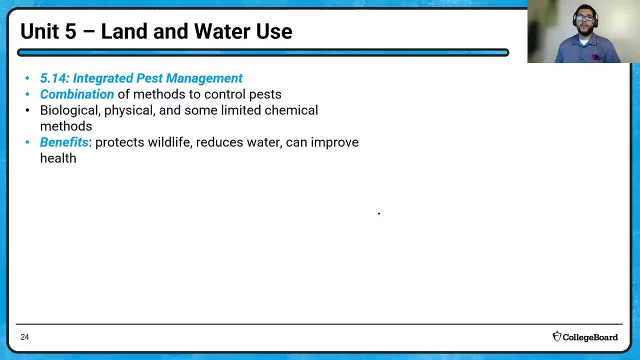 you can protect wildlife, you've got less water being used and, of course, overall health is improved. the downside is that it's a very complex system, it's expensive and it's time-consuming. right, i encourage you to look up cane toads and i guarantee you there's some really great. 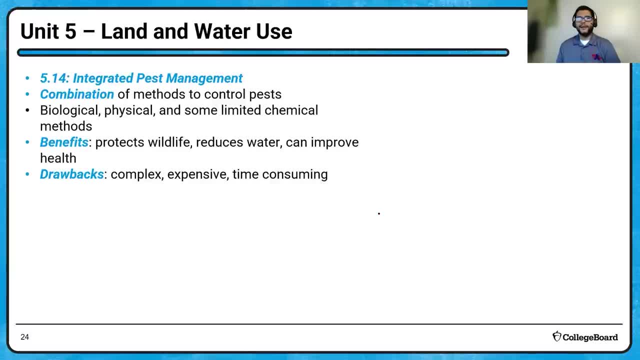 documentaries and some really entertaining ones on video services and stuff like that, and you'll be able to to see that there's sometimes biological controls that did not go so well. so that's cane, toads and all that stuff, and then you can use pesticides, and you can use pesticides and you can. 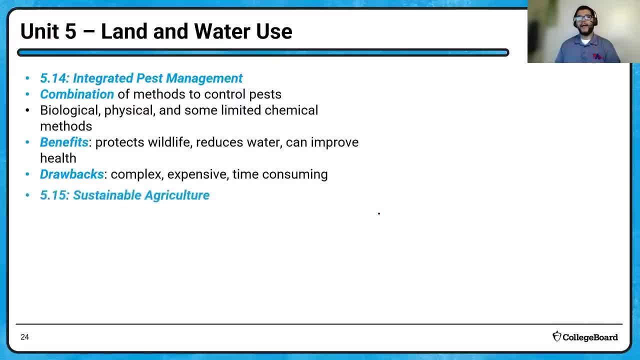 look for that one, and then you get sustainable agriculture right, so you want to be able to do this without having so much erosion right, and so we can do things like contour plowing, creating windbreaks, having crops that are more perennial, terracing, which is going to be a specific way of 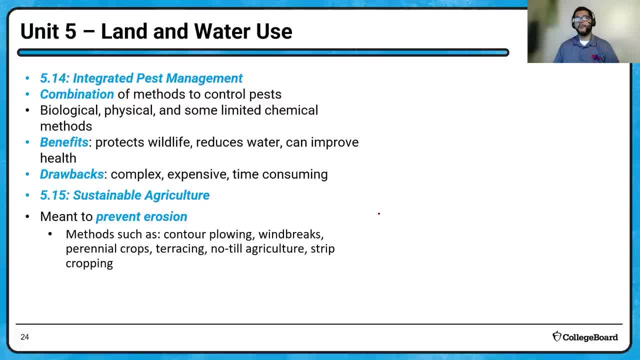 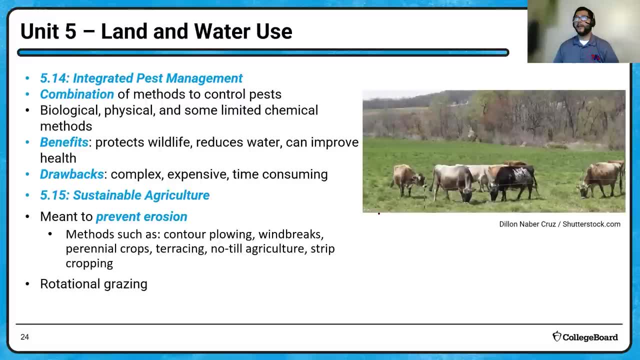 planting so that we end up not losing any water. and then of course, trying no-till agriculture or strip cropping right. and of course another big one is rotational grazing. so if you can have some animals like cows come in and graze, but then you move them from one area to another, then that 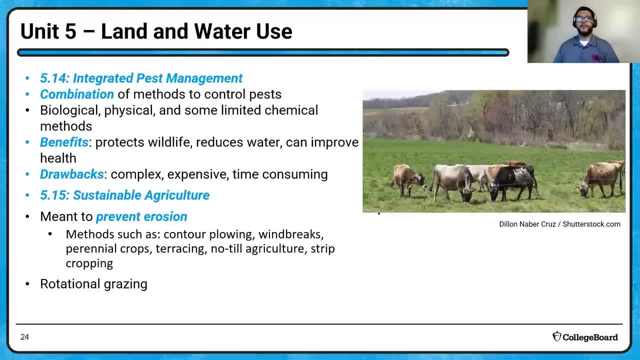 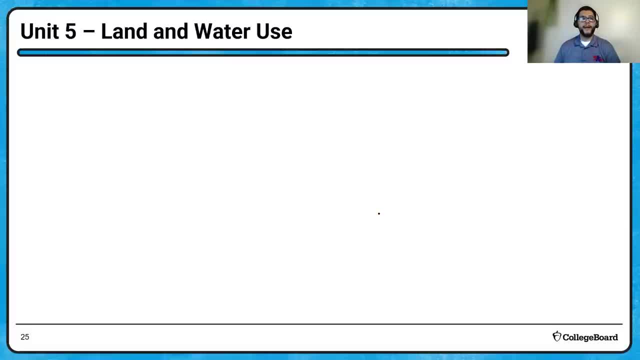 becomes more sustainable and they don't dry off an area, they don't cause eutrophication and erosion with their overgrazing. okay, and then finally last couple sections here of unit five, we get to aquaculture right. so one way we can prevent one of the tragedy of the commons with overfishing. 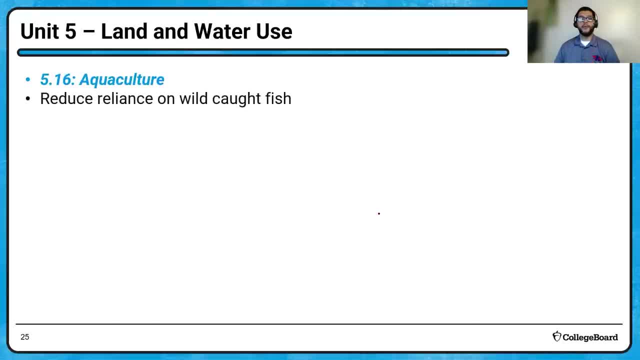 is maybe by growing our own fish and reducing our reliance on wild caught fish. so this is a current expanding adventure, right, and so there's a lot of great things. we grow our own fish. we have a food source ready available, but if, depending on how we do this, it can contaminate water if it's open ocean aquaculture. 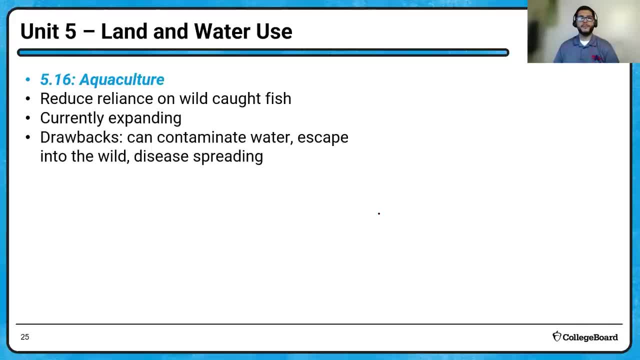 they can escape into the wild if you, you know, introduced a species that was not from that part of the ocean or that part of a body of water, and, of course, when you have a lot of animals that are in the wild, they can escape into the wild and they can escape into the. 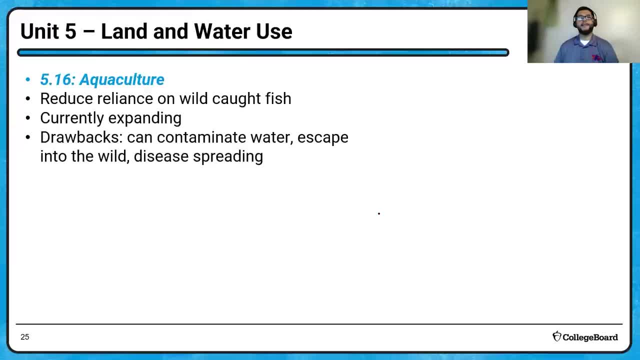 ocean. they can escape into the forwards and they can escape into the waters, and it's very interesting to look at when you're talking about other species like that. um, so we need to look at other species that are part of the ocean, and so i'm going to talk a little bit about the 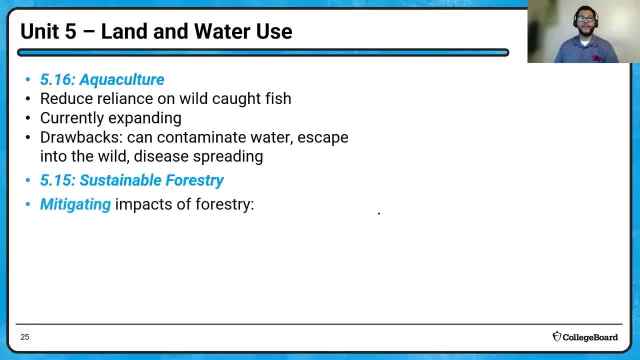 impact of logistic tools out there and how do we make sure that we are providing the right tools is a big, important term. that's where we take a problem that we created and we try to either slow it down or reduce the impact. so we've been trying reforestation, reusing wood, sustainable. 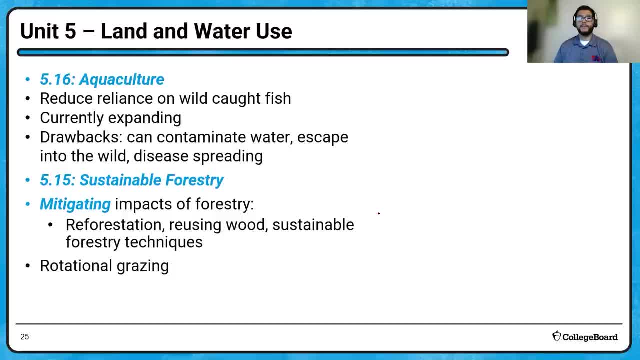 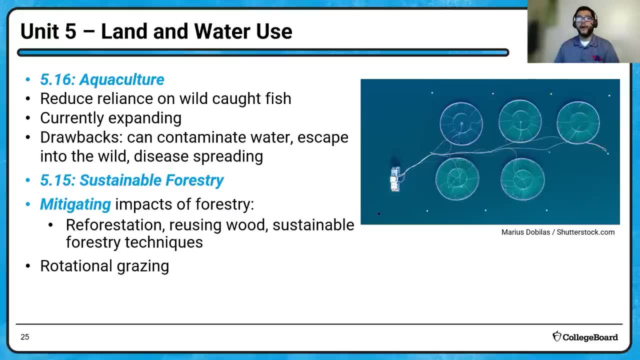 forestry techniques and also rotational grazing as well, so that we don't, so that we can have certain areas and not have to cut new ones down. and then, of course, you have those open, open, open ocean pens for uh land and water use, i mean for um aquaculture that can really impact our water, as 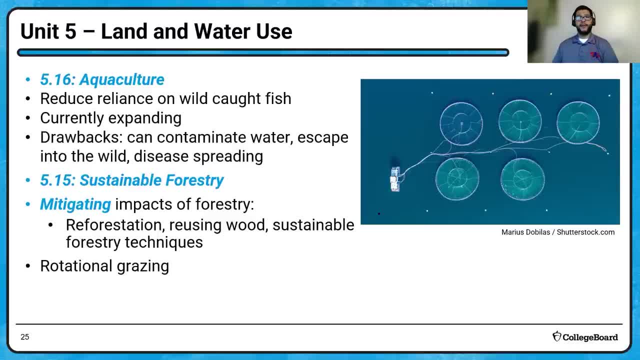 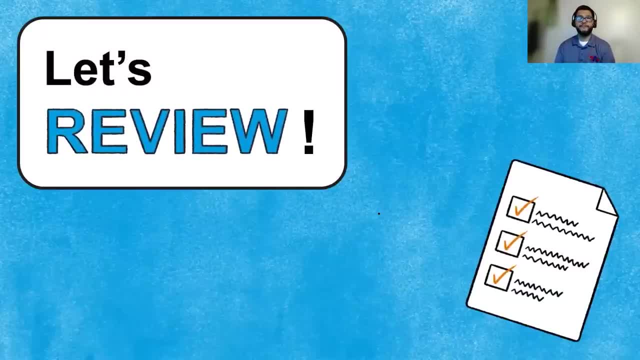 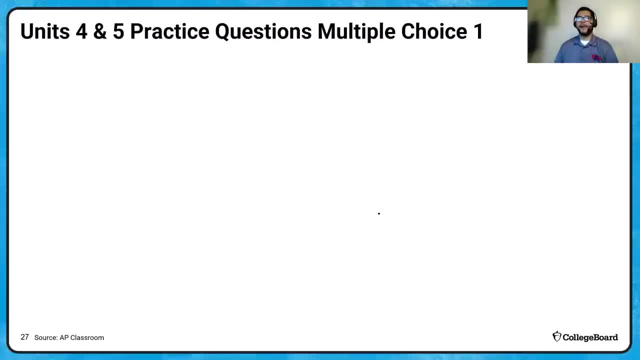 well, so that's a lot of unit five, and i encourage you, if there's gaps in here, if there was a topic you didn't hear from unit four and five, to please go back and review those right. okay, now let's go ahead and jump in to our multiple choice questions. so do some practice here. um, here is a question. 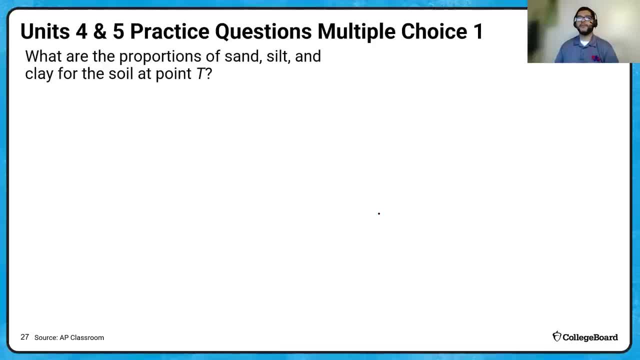 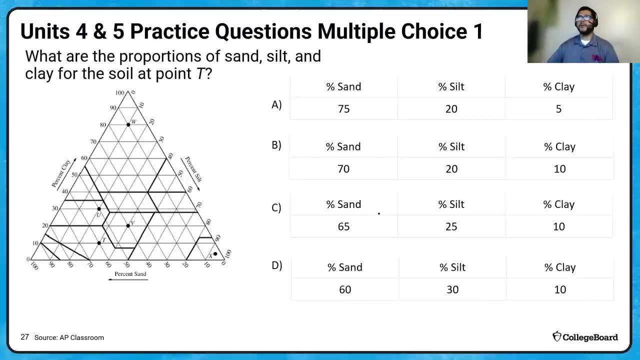 where it says: what are the proportions of sand, silt and clay for the soil at point t. so here we have a soil triangle with a bunch of points on there, and here's our choices: a, b, c and d. okay, now here's where we're going to end up with. 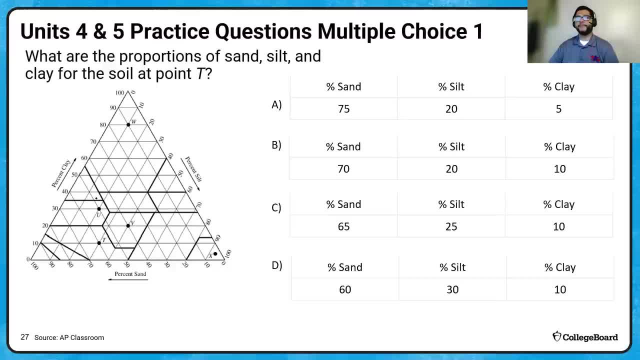 our uh, having to use our skills. so we talked earlier about using a soil triangle and making sure that we used the proper angle. so we start at sand, and what i like about this triangle is that they're kind enough, you can use the proper angle and you can use the proper angle, and you can use the proper angle. 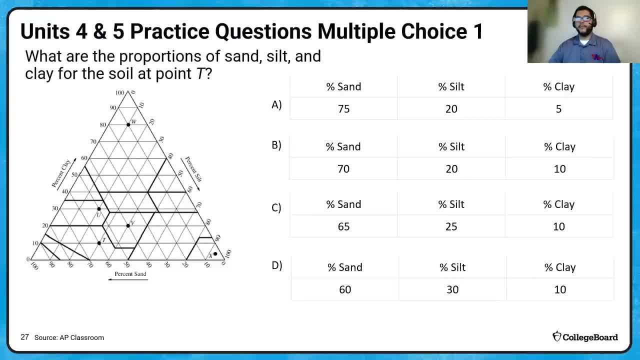 to already draw the lines in. so, if we look at it, the line from this t to sand is right. here it's the 60 percent line, okay, so we're good there. now we pointed it towards clay, and now for this one for clay, we need to point that towards silt, and to the point. we're going to remember this is always a. 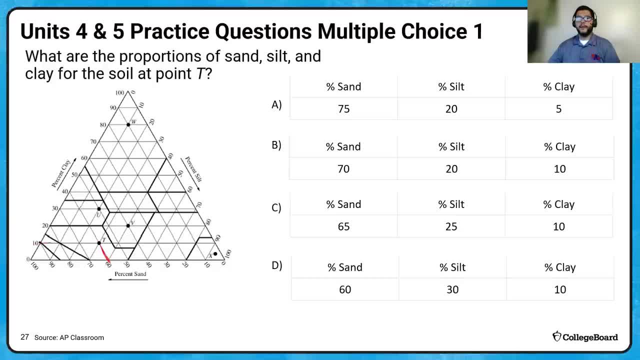 horizontal line. so that's going to be right here. excuse me, it's going to be right there, okay. and then for silt, we need to take the point on the edge of silt and point that back towards sand, and that line is right over here. so sorry, if it's not too straight of a line, my bad. and then if we look at, 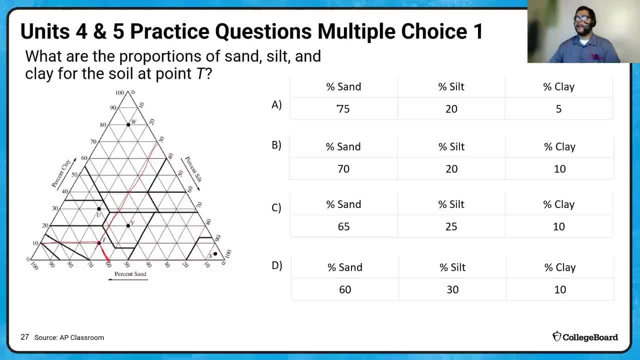 it 60, 10, 30, so sand 75, 70, 65, and then there's 60 right, and then for clay there's 10, 10, 10, so it's either one of those three, and then for silt it's 30. so our answer should be, in this case, letter b. 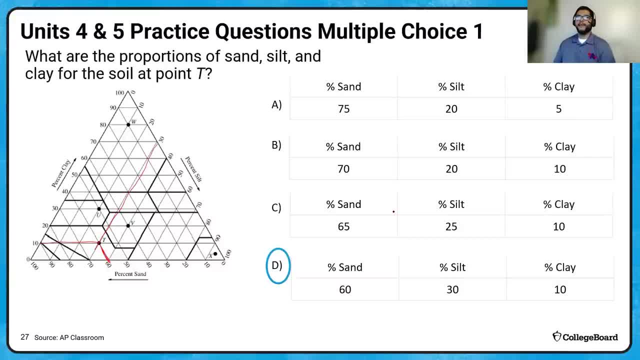 okay. so if you get a question like that, that's awesome, right? um, i know people look at these triangles and they're. they always have this moment of panic like, oh no, i don't know how to use this. i'm confused. remember our strategies from video one. if this looks like it's too much work, or you. 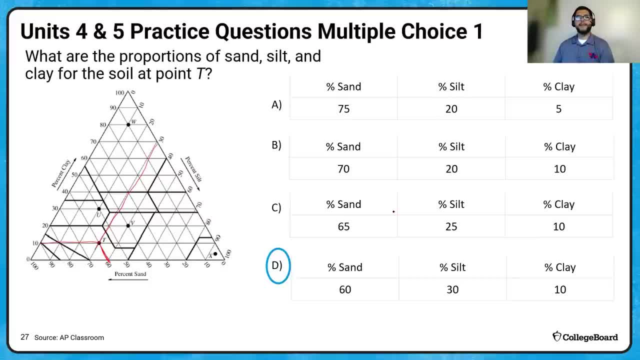 have to overthink it and it's going to take you too much time. make it a second round question. come back and hopefully you know how to do this, you're paying attention and you can go. all right, let me go ahead and review this and try again. 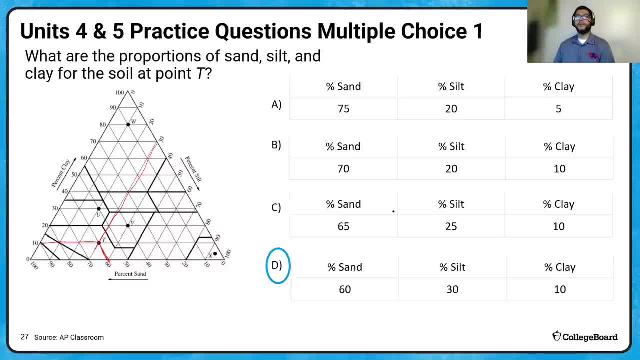 or if it's to a point where it's just too much, you can make it a third round and just give it your best guess. now here's what i would have done if i was a little unfamiliar with this. i would have just tried to connect one of these right, so, like if we look at sand, and connect one to that. 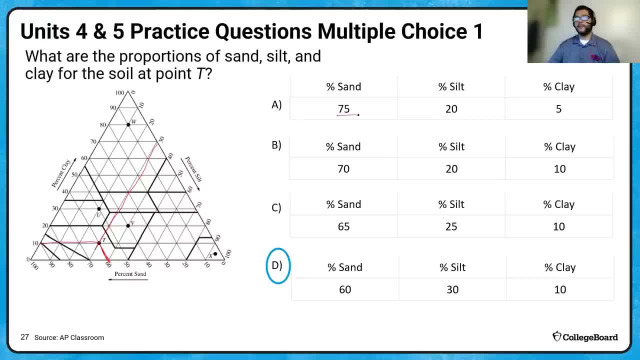 letter t if you look at the rest, 75, 70, 65 and then 60. so it would have been a pretty easy giveaway if you just identify sand on this one. so always look for what you can right, look for whatever angle you can to try to answer these. quite literally, an angle here. 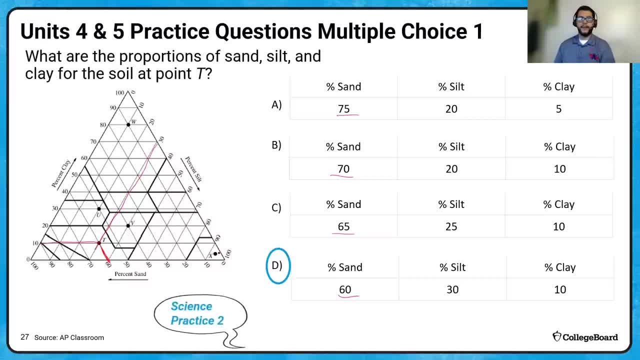 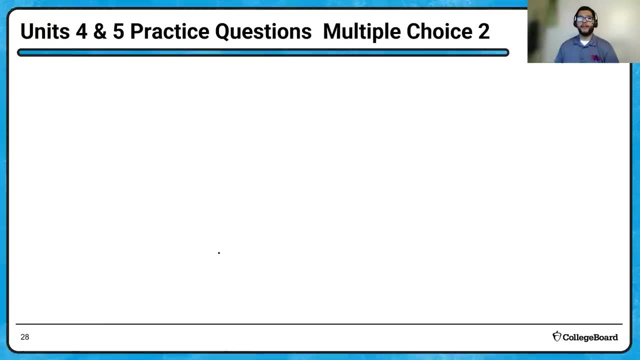 and so this was science practice number two. right, and also don't forget to go back and review unit four, uh, soil composition, soil properties, um, and soil triangles- right, okay, so now question number two. if we take a look here during an elenio event, warm water surface. warm surface water moves from. 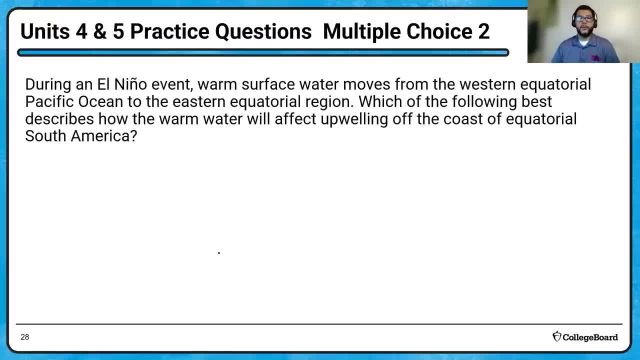 western equatorial pacific ocean to the eastern equatorial region. which of the following best describes how warm water will affect upwelling off the coast of equatorial south america? so some big words here, upwelling, um which ocean? we're at, and it's an. 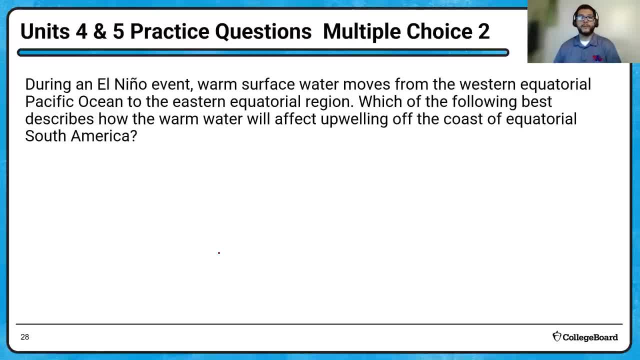 elenio. so that's going to be that, that unusual warming? so is it? warm surface water will not change upwelling, because this region is at the equator and always has warm water. the warm surface water will increase upwelling because the difference in salinity between the warm surface water and the cold deep water. the warm surface water will decrease upwelling because the cooler temperatures on land in the region will prevent upwelling. or is it? the warm surface water will decrease upwelling because the density difference between the warm surface water and cold deep water. so, if you want, 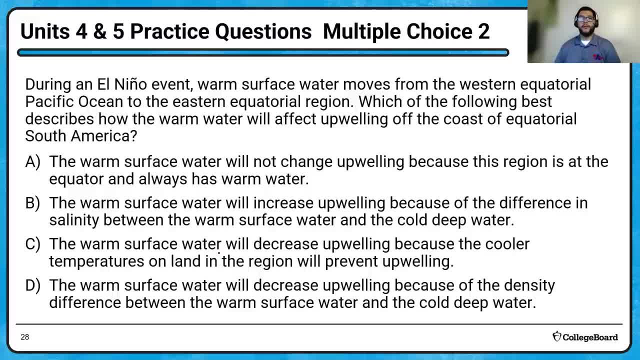 take a minute, think about this one and give it a shot if you want to pause it, but if not, the answer should- in this case should- be d, because that's what causes it. right? you end up with a change in density and so because of that change in density will decrease upwelling because the cooler temperatures. 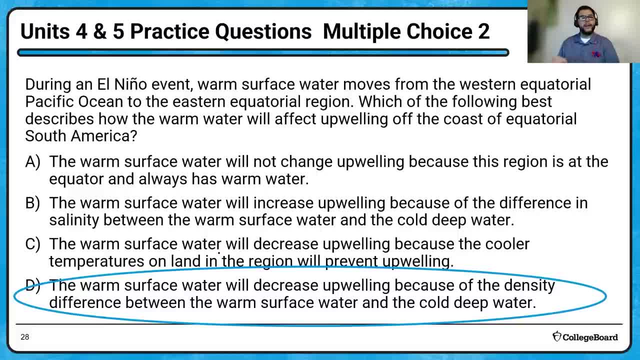 and the density that cold water doesn't get to come up anymore. it doesn't well up right, and so that ends up causing this um warm spot and that's why you end up with poor fishing off the coast of south america. okay, and so this is a practice. seven, so identifying environmental problems. 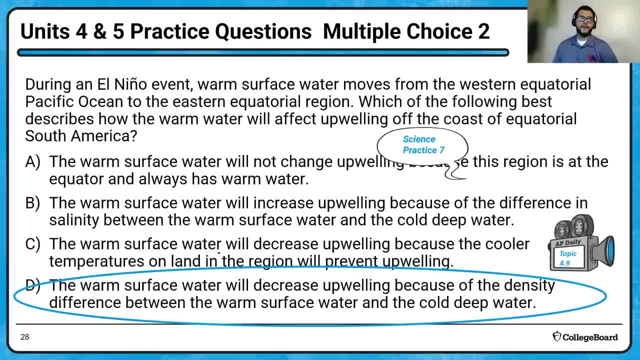 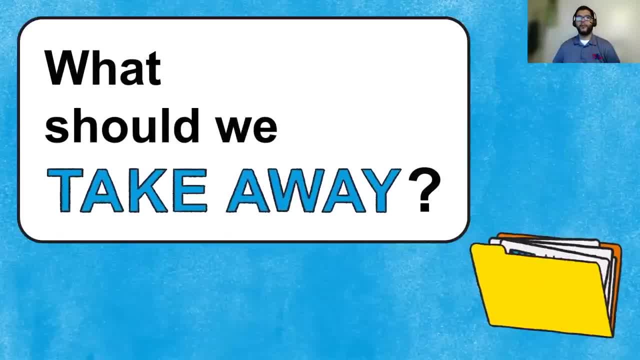 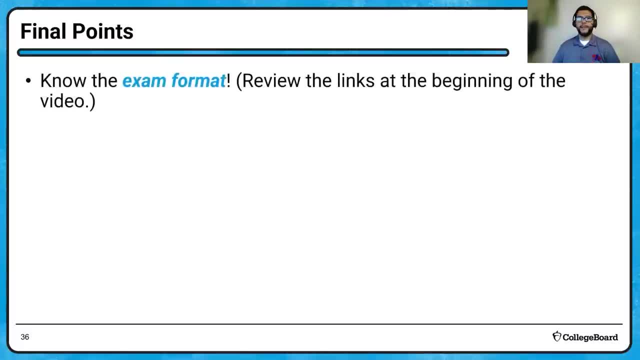 and, of course, make sure you review. the el nino topic is on the on this one. so that's all for me, right? so what are what? should we take away? some big final points here, right? obviously, as i've mentioned before, make sure you know the exam format. review those links at the beginning. 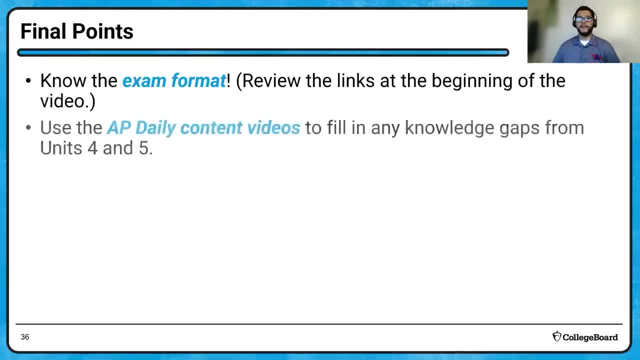 of the video and then check your ap daily content videos to fill in any of these knowledge gaps in unit four and five. so if there were things that we didn't go over that you want that you need to go look at, go to ap daily. they will help you, though. they will help you with those, because this is not 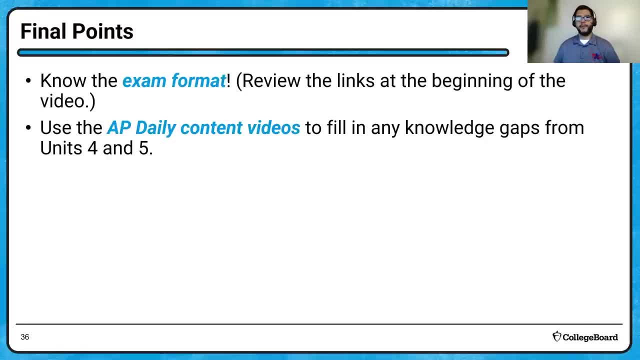 a long enough format for us to go over everything in those videos and then, of course, prepare to go in in depth into those topics and the units they're going to be in there and then, of course, practice these topics because they're the toughest for students, right, um, and you can also apply the solutions. that's the big important.